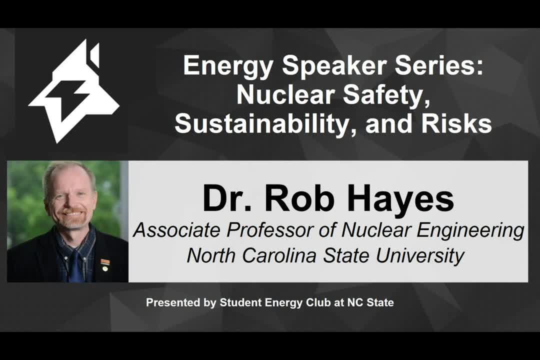 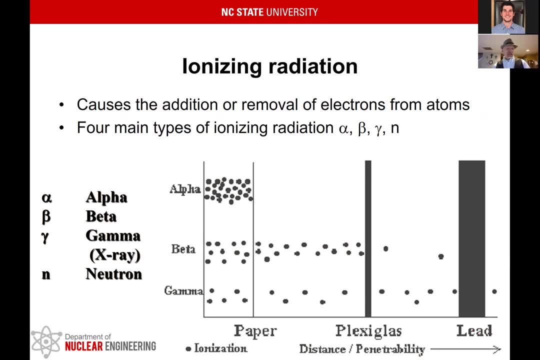 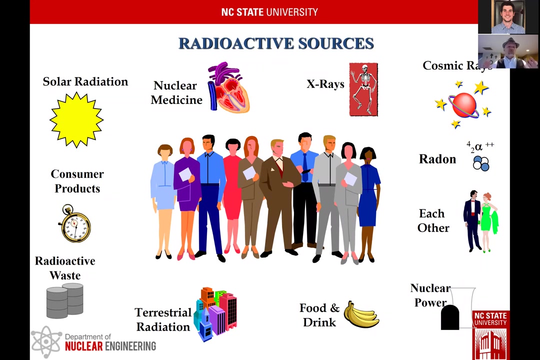 Thank you. In fact, the actual source of energy from geothermal is radioactive decay in the core of the earth. All of the primordials, the uraniums and the thoriums and the potassiums, those were here at the formation of the earth and they're still here, And their decay inside the earth keeps it molten. That's where the heat comes from. But the point that they're primordial means that they were here at the formation of the earth And they'll be here even after the sun goes red giant. They'll still be here And so they're everywhere And they get concentrated in different places, just like other ores do, like, you know, iron ore or nickel ore. 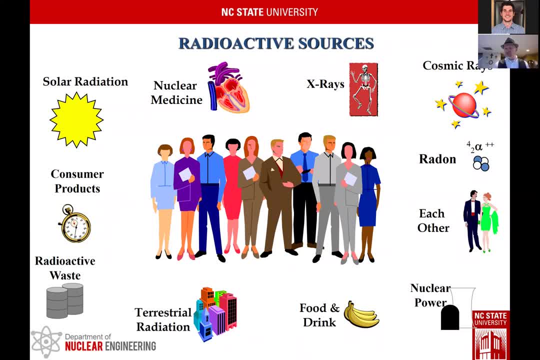 Or something like that. But because of the potassium it also gets concentrated in food as long with other things like radium or other radionuclides, can get concentrated in foods And they're also used throughout industry. There's some pictures here of different places where you get them. Now they're not all equal. They're going to give very different doses. What we'll find out here shortly is the radon. in terms of these, and medical are the big ones. 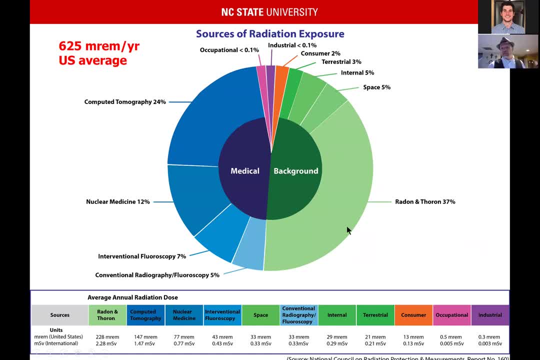 So you can see here that, from the background, all of this stuff that's green over here, this is natural. This is what you get just because you're alive, right? Because you're not shielding yourself from the earth And because you're not wearing a filtered mask and you're breathing in radon, And because you're not deep underground- you're not shielded from cosmic rays, right? All of this over here is what you'd get just because you decide you want to live in the biosphere. So that's what's natural. 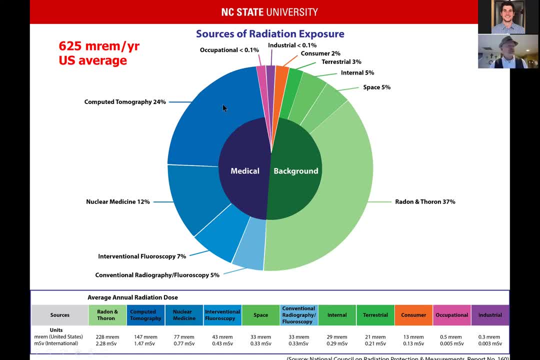 What we get over here is the benefit from medical, Basically a doctor's ability to see if your bone is broken, so they know how to set it, so that they can do fluoroscopy, so that they can do some kind of an intravenous procedure. 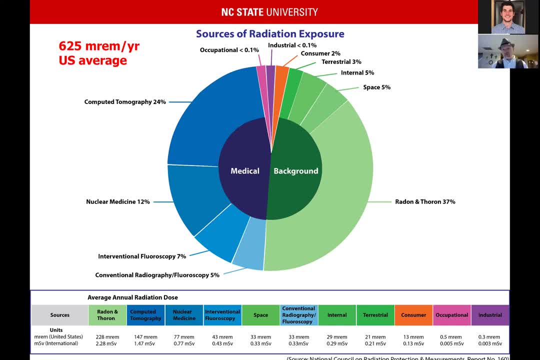 Without having to cut you open. you can do basically outpatient surgery Instead of having to, you know, do a two week's stay because you got your torso cut open or something like that. And so, on average, this is about 625 milligram per year. when you take in the background and the medical- Now typically medical x-rays- you get more of those as you get older. 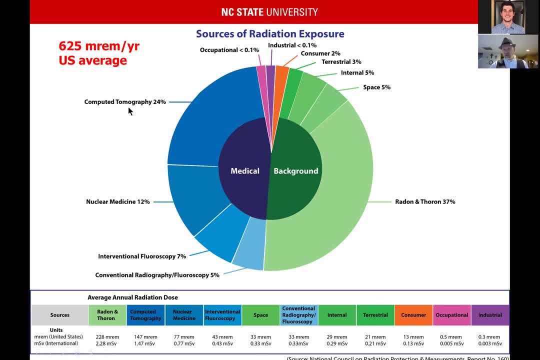 but it will all depend. But this is just the US average. That kind of scales with what is ambient in terms of your damage, day-to-day exposure from both background and medical. Something that I'll point out here is that for industrial that's like nuclear power or other kinds of things that have to do with 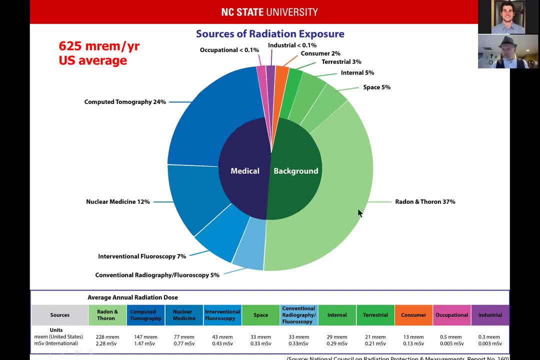 nuclear technology, And this is all going to be less than one-tenth of a percent. A lot of it's going to be even a smaller sliver of that. So you have to basically lump all of them together just to get that tenth of a percent. You can see it's even less than that. So what we do in health, 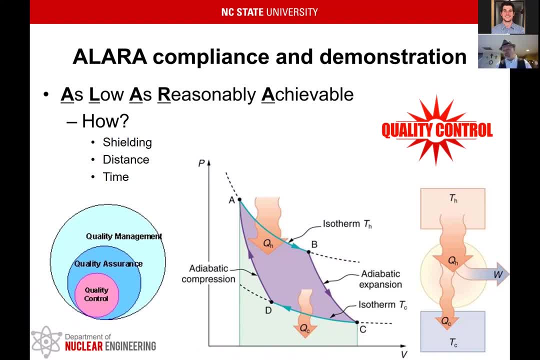 physics is largely ALARA And that means we're just controlling radiation, And the ALARA program is really like a QA program. If you were making widgets, let's say you're making phones, or you were making coffee cups, or whatever you're making as an engineer, you're going to want to optimize. 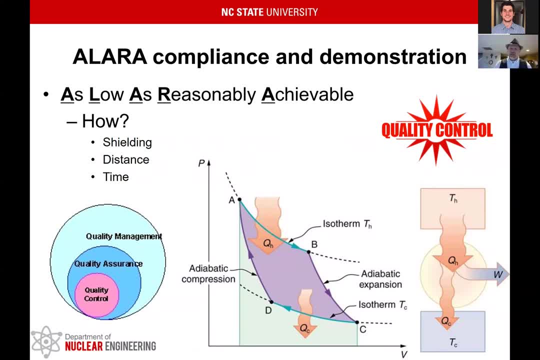 the process. You're going to want to minimize waste, You're going to want to minimize energy, You want to increase throughput, You want to increase quality, And all of these things require tracking and trending, which is really what ALARA does to make sure that we're in control of all of. 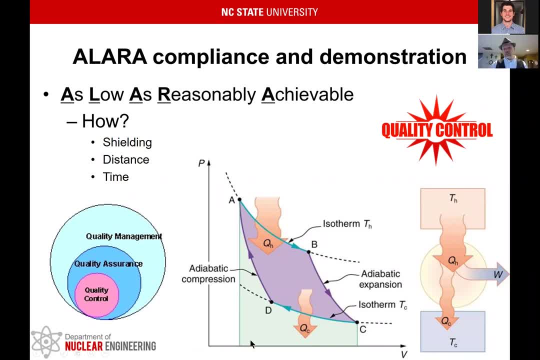 the radiation and the radioactivity. And so, just like when you're doing heat theory, heat combustion theory, there's a limit to how much you can get. when it comes to thermodynamics, You have the Carnot efficiency, But as an engineer, 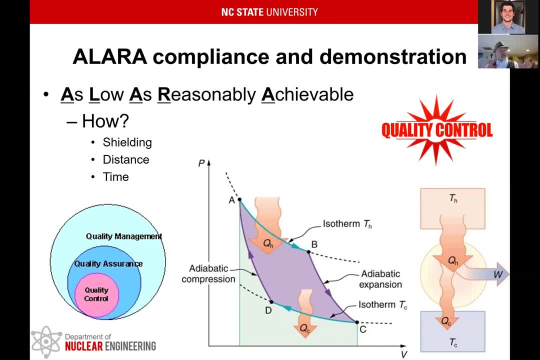 you're going to want to get as close to that as possible, But by the time you're right near 40%, it doesn't make sense to spend another million dollars to get a tenth of a percent right. It's a balance of how much it costs to get to the highest efficiency, And so that's a risk management. 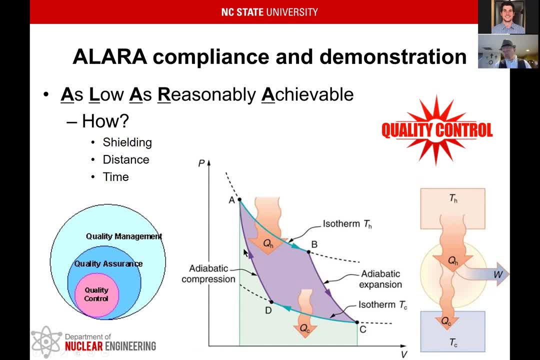 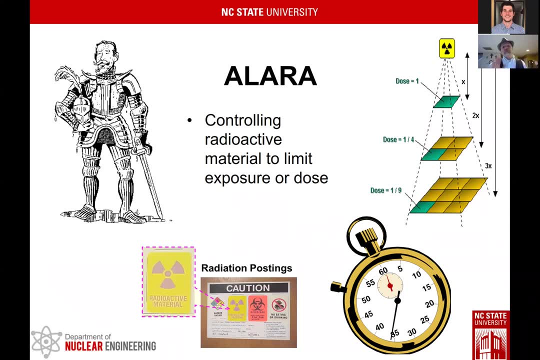 issue that we have Both in the nuclear industry and in every industry. you want to do risk management. So with ALARA, largely the biggest focus is on shielding, on postings, basically letting people know: oh, there's radioactivity in here, You can't eat in here, You need to wear PPE. Minimizing the 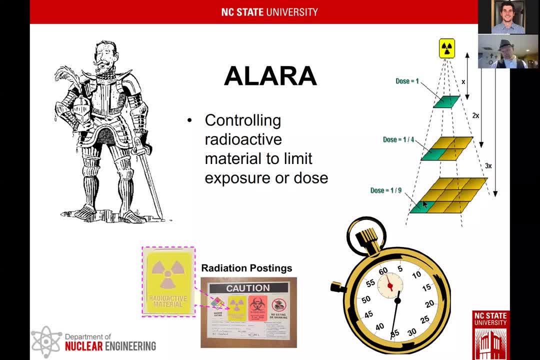 time when you're in those fields, And then recognizing the distance effect of inverse square, meaning that the radiation attenuates as the square of the distance. So if I double the distance, the radiation field goes down by a factor of four. It's the same thing with a light. 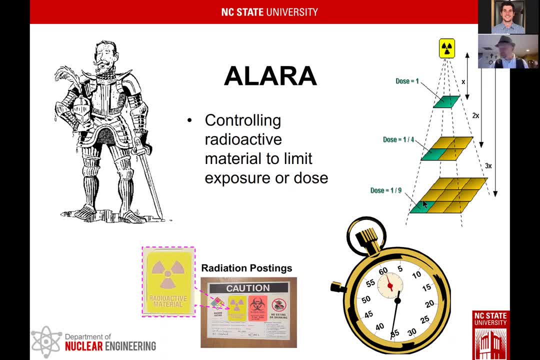 right That the intensity of the light goes off as one over R squared. Or gravity does that, Or a Coulomb field does that. It's an inverse square dependence Because it's uniformly distributed over a sphere and that sphere area is proportional to the square of the distance of the radius. 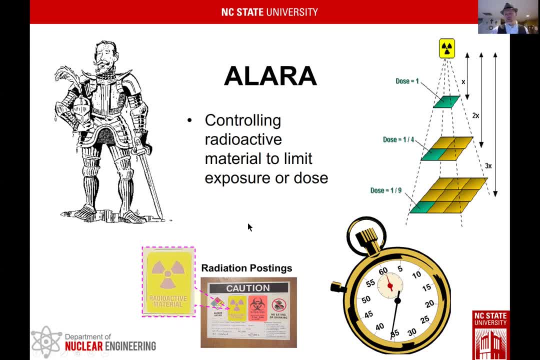 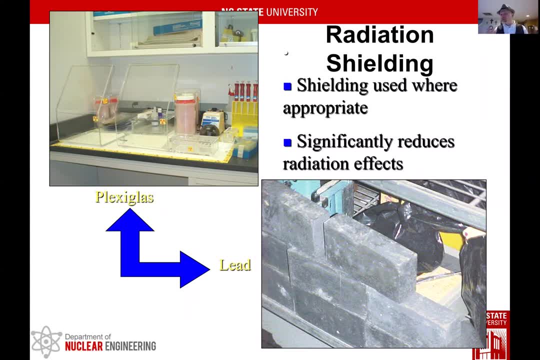 And so that's how we do ALARA, how we control radiation fields. The bulk of it is those kinds of technologies. Here's some examples: This is a medical facility where they got some beta radioactivity that's being used for nuclear medicine, and just plexiglass. that's all you. 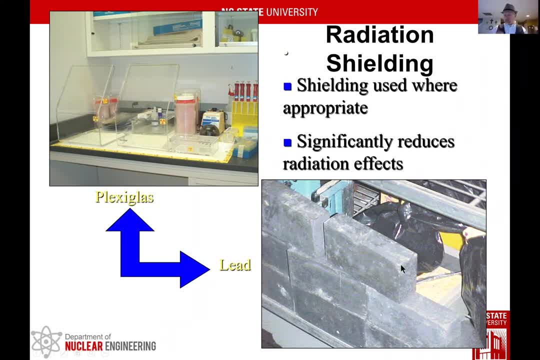 need to shield the beta, but if you've got gamma, then we can use lead bricks or concrete or something like that, because you need something with a high density and high atomic number to really attenuate those photons, those gamma, those high energy photons. now, when it comes to these, 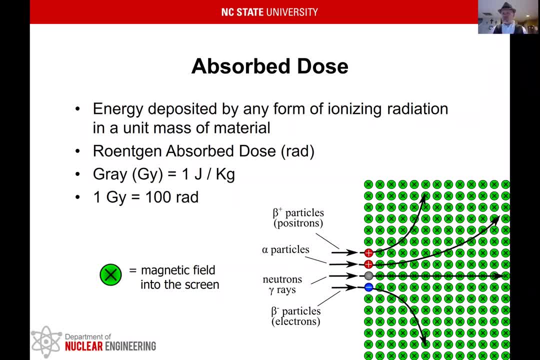 kinds of radiation. they interact differently and what we're always concerned with is the dose. when it comes to any kind of radiological risk, the risk is going to be in the dose. so there are other kinds of particles. you can have neutrons, uh, and you can have positrons as well, and they're going. 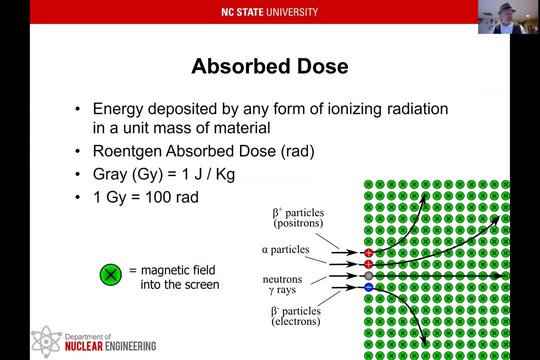 to behave differently depending on the environment that they're in and the way that they interact. but what they all eventually contribute to is this number, this energy per mass, so that the dose is an energy deposited per mass. that's the dose. how much energy in a material? uh, did you? 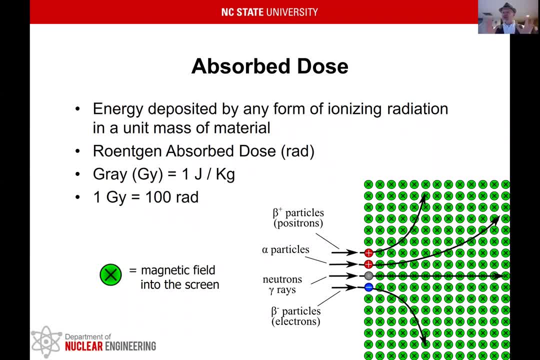 deposit divided by the mass of that material, and that's going to be the, the dose, the radiation dose that it received. And even though each of these will interact in a different way, it always comes back down to that same parameter. What was the energy per mass? 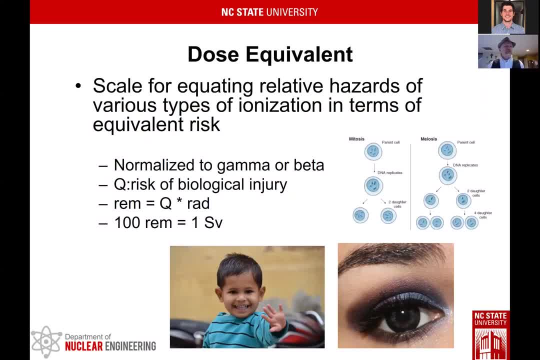 Now we have something else that's called the dose equivalent. The dose equivalent is like a radiological effectiveness in terms of biological damage. So if you have any kind of high proliferant cell division, that's going to be more sensitive to radiation. Children are more. 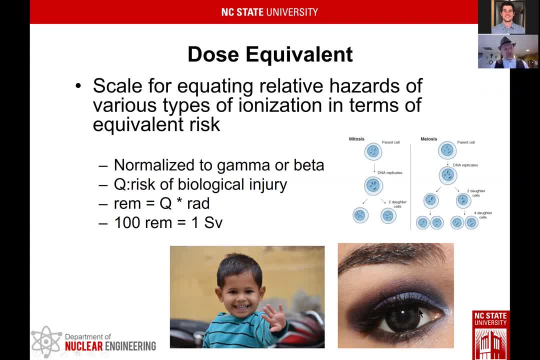 sensitive to radiation. Highly ornate pieces of the body are more sensitive to radiation, So that the eye is going to be more sensitive than, say, for example, the nose, And the gonads are going to be more sensitive than the phalanges. The more detailed the biological mechanism is. 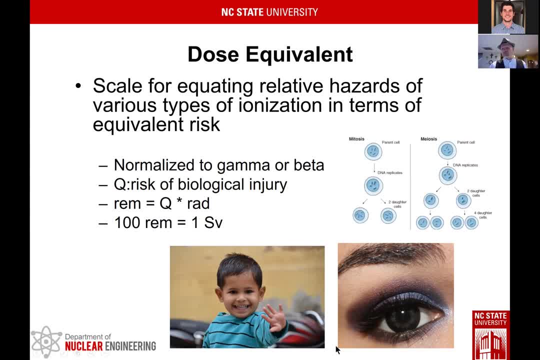 the more sensitive it's going to be. And so then we convert from the energy per mass to the equivalent energy per mass, And then we're using REM and Sievert, which folds those kinds of things in. Now, when it comes to just beta and gamma, one rad will equal one REM. 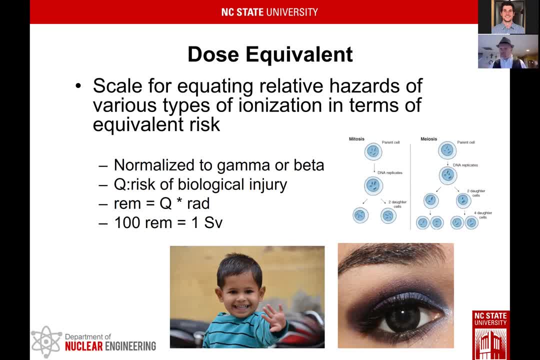 and one gray will equal to one Sievert, But in the United States we largely default to REM, simply because that's what the regulations are written in. The regulations are written in these American units, so to speak, CGS, as opposed to SI, where the Sievert is the SI unit. 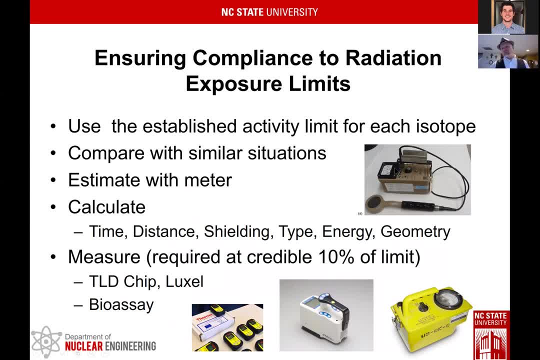 So the way that we measure these are with a little bit of a scale, So we're going to hand-held. I'm sure you've seen some of these in like in Hollywood: different radiation detectors. These are what we use to measure radiation fields. You can't see it, smell it, taste it, So you. 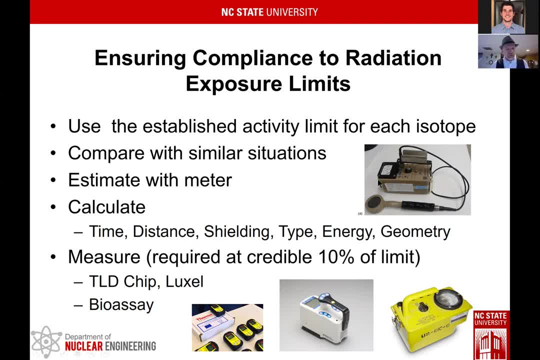 actually have to measure it. It's kind of like an electric field. You have to have an instrument to measure it. I've seen in Hollywood that what you see here, this part of the this, is a Geiger-Muller tube. This part right here is the active part, And I've seen people using it upside down so that 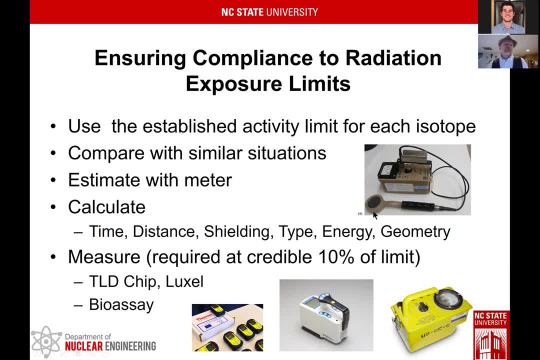 they have this point, this surface, pointed up, And in Hollywood they don't know, And people that are watching it probably don't know either. So it's kind of fun to watch. You know they've got the instrument upside down, but nobody knows any better because 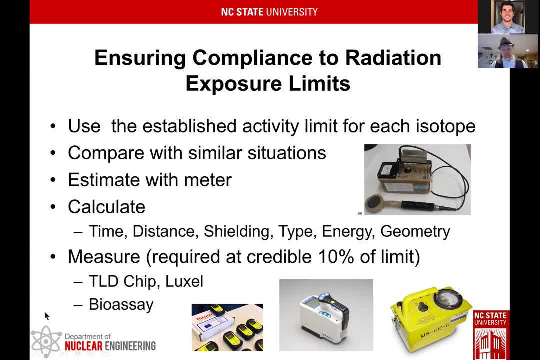 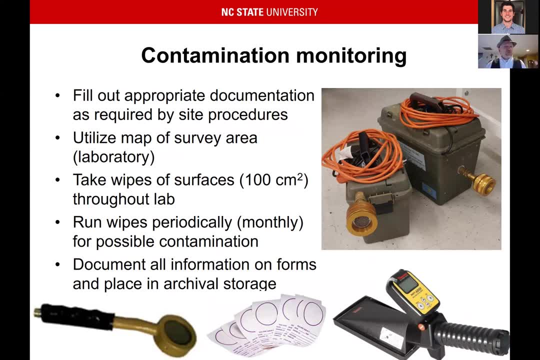 none of them have used it, But we also have other techniques as well, such as TLDs. So besides measuring just radiation fields, we also want to look for contamination. So these are air samplers. Basically, this is a pump and you pull, you put a piece of 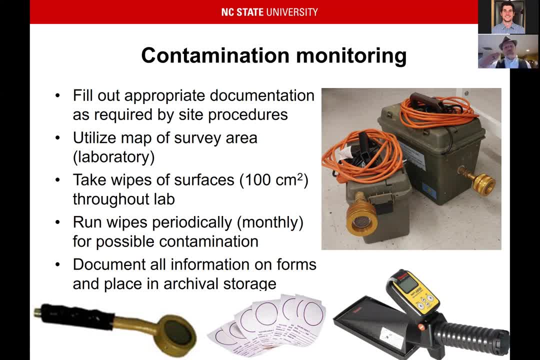 filter paper on that nose of the pump and then you pull a known volume of air through that pump. After you've done that, then you'll take that filter paper off and you'll measure with a device like this or some other kind of a device, And then, when you measured the activity on the filter, 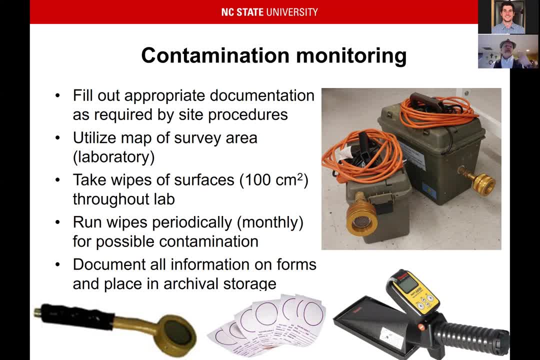 you divide it by the volume of air that was pulled through it. That ratio is the concentration of the air that you ascribe to the volume that you sample, And that's how you would measure air contamination. Alternatively, if I had a surface say, for example, it was my phone and I wanted to. 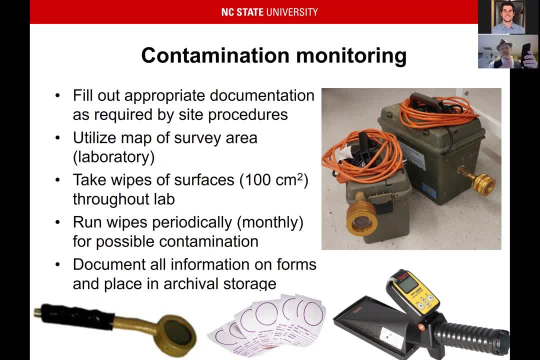 know if there's any contamination on the phone. I could use one of these hand-helds and just put it right up against my phone and see what the total amount of contamination was on the phone. Alternatively, I could take one of these smears. Basically it's a piece of like a filter paper with a sticky back and I can fill out some information on the back. 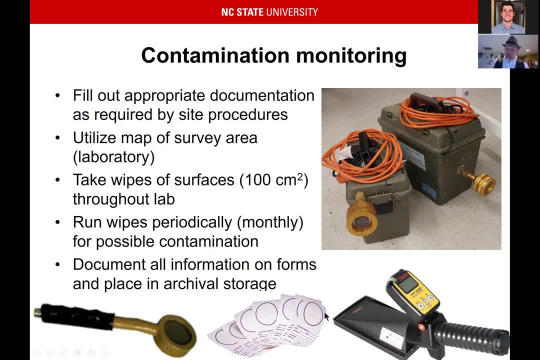 And then I just rub it over the surface of my phone And then I take the smear to one of these handhelds and I'll measure the smear and see if there's any contamination on the smear. We call that removable contamination, Whereas if I just took the detector and put it up against the phone, I would call that total. 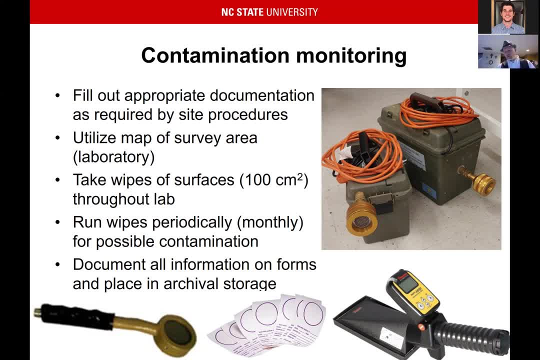 That's going to be the removable plus the fixed, And so that's how we would measure both fixed contamination or airborne contamination. So that's pretty much the kind of way that we characterize an environment: the amount of contamination that you have and the radiation fields that are present. 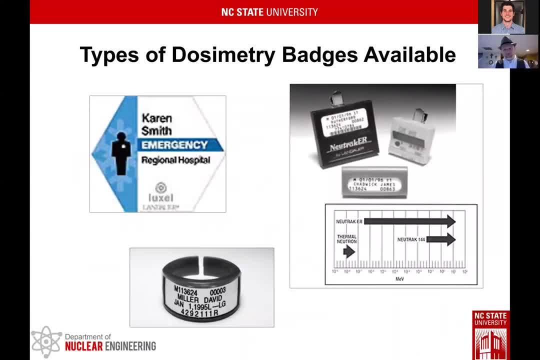 And they can both be very well, very intimately, related When it comes to personnel dosimetry. we're going to have them wear a badge. These badges will have little crystals in them that will absorb minuscule amounts of energy When you deposit the energy into these crystals. 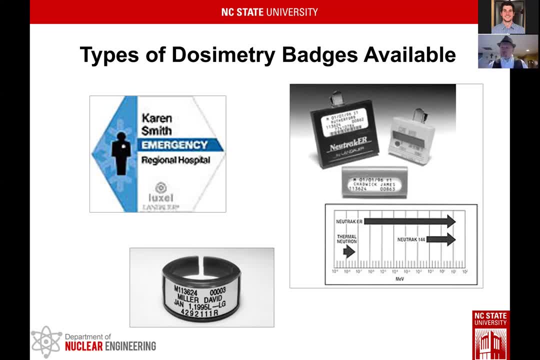 From radiation at defect sites. they're going to be able to absorb a little bit of that and retain it, kind of like a glow-in-the-dark frisbee will retain some energy when you shine light on it. These crystals here will retain the energy a lot longer. They can be read out later to determine what the radiation dose is, once they've been properly calibrated. 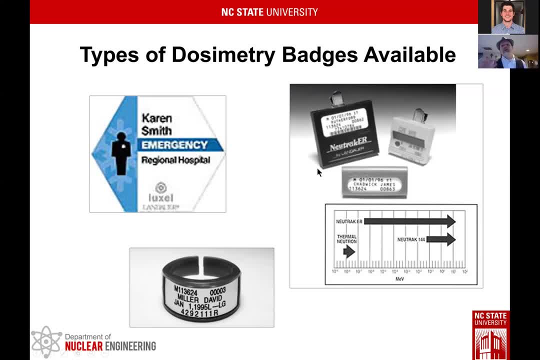 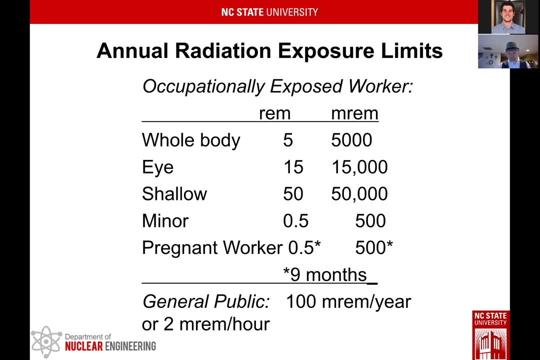 And you can have a ring dosimeter or a torso dosimeter or any other kind of dosimeter that might be of interest for characterizing historical radiation fields that a person was exposed to. So, when it comes to the regulation, These are what's considered the law. 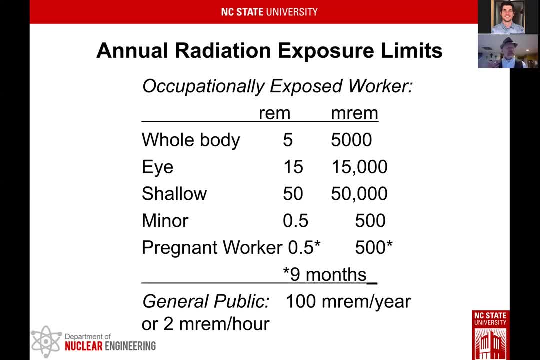 So these are in the for any of the federal facilities or any facility that's regulated by the Nuclear Regulatory Commission. You can see the maximum dose that a radiation worker can get is 5 rem. That's considered to be comparable to the OSHA limits for other industrial activities. 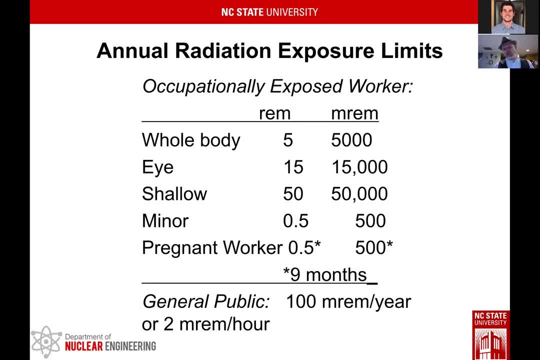 And this assumes what we'll talk about just a little bit, called the linear no threshold hypothesis, Such that if you have a safe workplace, that if you're getting 5 rem or less, That's considered safe. Typical nuclear facilities will have nuclear workers getting on the order of about 100 millirem per year, less than background. 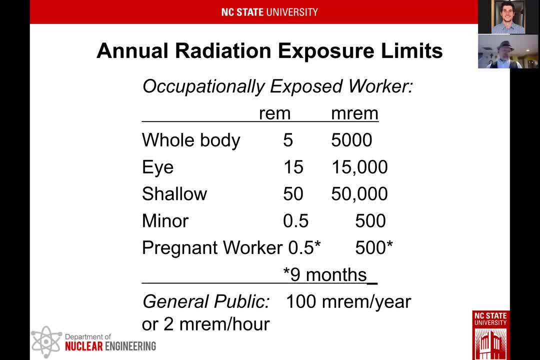 That's not unusual because it's not that difficult to control radiation fields when you're actively doing that. Most facilities will have an administrative control limit. that's on the range of about 2 or 1 rem. So you can get substantially lower than that. but that's just the law. That's the maximum that you could do. 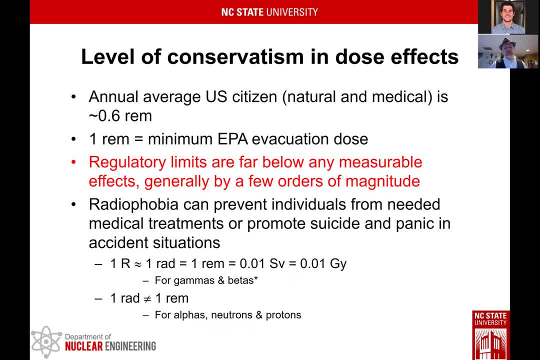 Well, let's look at this in terms of actual measurable risk. So again, I showed you before that it was about. it was just over 600 millirem that you get from all sources combined. Now to put this in perspective, in terms of regulations at 1 rem if there was a large contamination event. 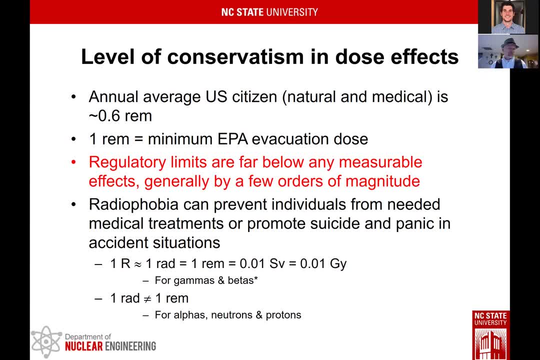 The EPA would issue recommendations that everybody move away from their homes and evacuate if they could get as low as 1 rem per year. Now the maximum is 5 rem, but the point is is that that's where they issue that recommendation, at the 1 rem level? 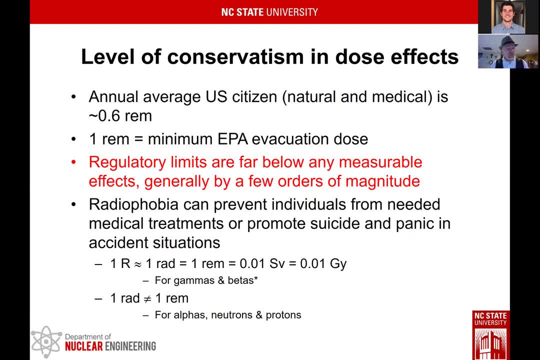 And so this can kind of feed into what we call radiophobia. People think if you're making me move from my home, it's going to have to be incredibly serious if I have to move away from my home, even though this is in the safe limit. 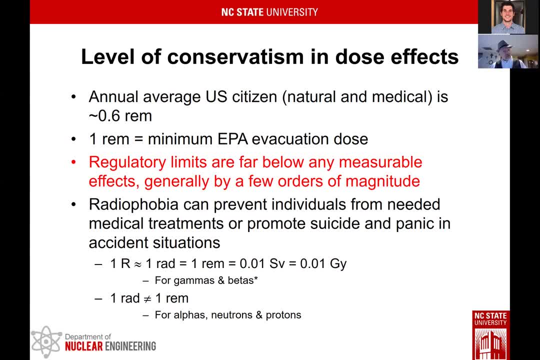 It's just that they're being that protected. That's the idea. Remember, children are more sensitive and they don't want you getting lots of vectors right. So if you're getting 1 rem from 5 different places, suddenly you're getting 5 rem. 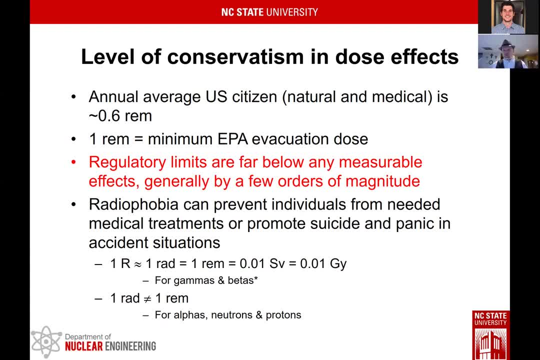 And so that's the way that they think about it. even though you recognize that this is a dose that you legally could get for a radiation worker, It's substantially lower than it, And so it's difficult for a lot of people in the public to be able to discriminate between what's safe and what's scary. So let's start looking at that a little bit. 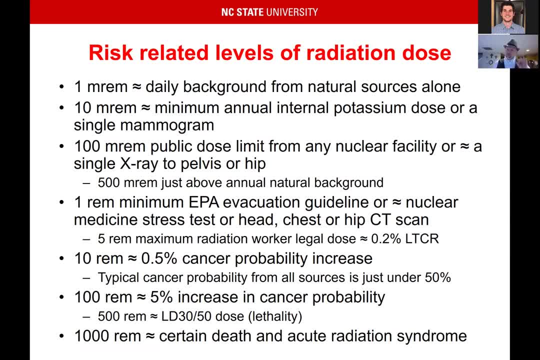 In terms of your daily background dose, that's about a miller rem. Remember it was about 325 miller rem per year, So that's about a miller rem per day. We're just going to go through orders of magnitude here until it actually gets scary. So 10 miller rem, that's about what you get annually. 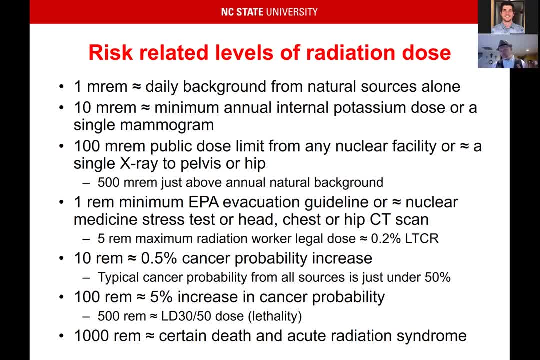 if you're very, very small person, just from your internal potassium. Remember, potassium is essential to live. You will die without it. The sodium potassium pump is what gets water in and out of cells, So you have to have potassium to live. 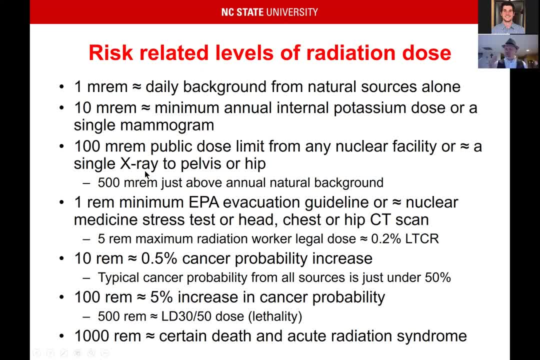 And you'll get. and potassium is naturally radioactive, So you'll get about 10 miller rem. or a large, muscular male might get 40 miller rem. a small, petite female might get around 10 miller rem. It scales with muscle content, the potassium that's in there. 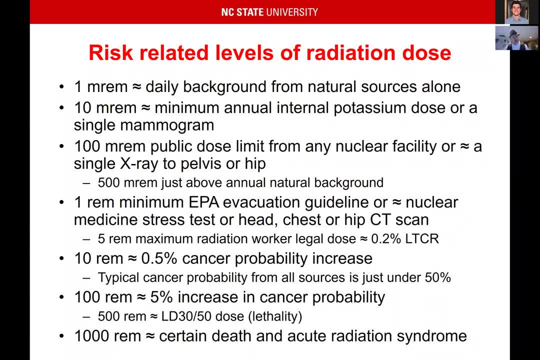 Going up a level, the 100 miller rem. that's again less than background, Annual background. but that's about what you would get from a single x ray to your pelvis or hip. It's also the limit for the public to a nuclear facility. That's the maximum the member of the public can get. 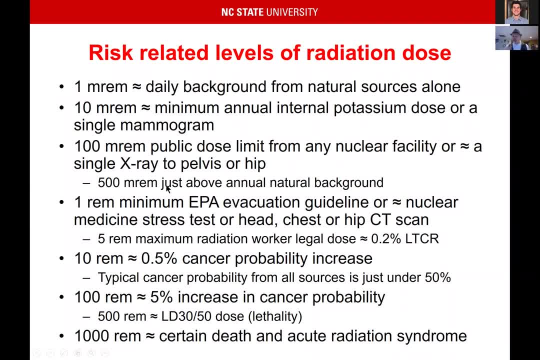 Now one rem, that's the EPA evacuation dose. That's about what you would get if you were to do a stress test- I've done one of those where they look at the functioning of your heart- or if you were to get a CT scan of your hip or chest or your head. That's again around one rem. 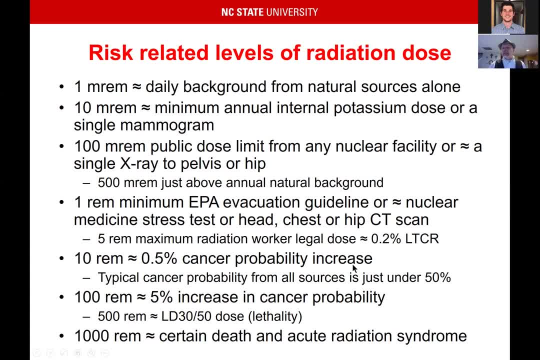 Where again the five rem is the maximum radiation worker And at that level, at five rem, it's about two tenths of a percent. that's assuming the linear no threshold. two tenths of a percent increase in your lifetime cancer risk. 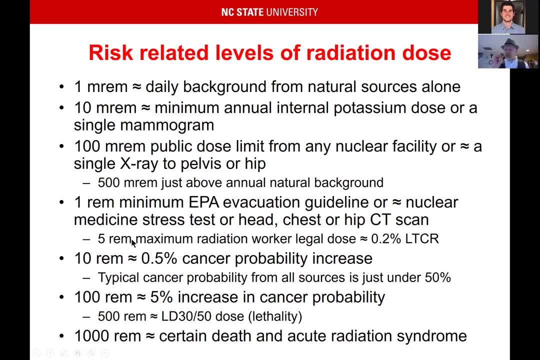 It's not until you get to 10 rem that we just start to get where some studies have been able to claim that they've seen an increase in cancer risk, And there it's about half a percent. And the reason why you've got to get to that big of a dose before you see anything is because your ambient cancer risk is already between about 40 and 50%. 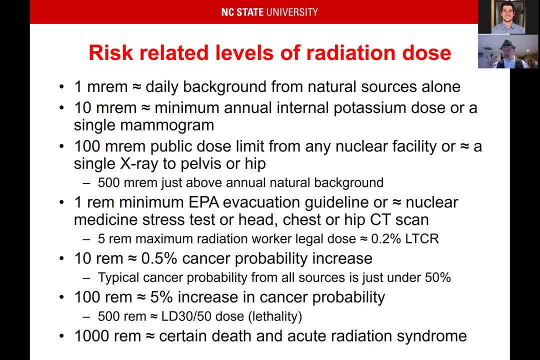 Just for the average citizen, And so to be able to see a statistically significant increase, it's going to take a large relative increase in order to see that, And that starts right at 10 rem. The majority of the papers don't put it out until around 20 or 30 rem. 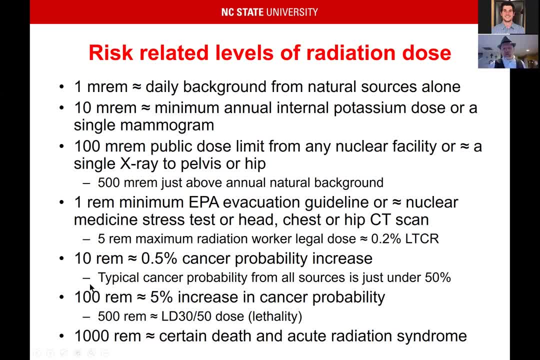 But all of this is based on the atomic bomb survivors who got doses around 100 rem, 100, 200, 300 rem, 50 rem doses like that, And when you're up in that range, the probability increase is going to be about 100 rem. 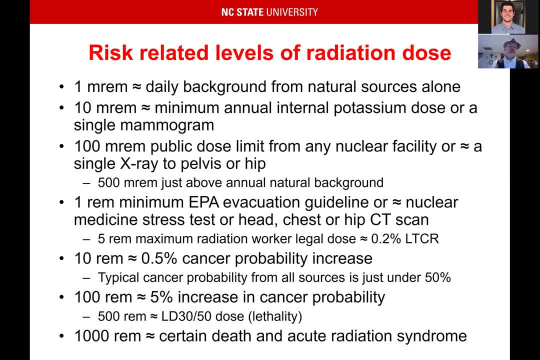 And the probability increase from cancer due to dose is linear. So if you double the dose you double the probability of getting cancer, so that at 10 rem- or sorry, 100 rem- it's around 5%. So at 200 rem it would be 10%. 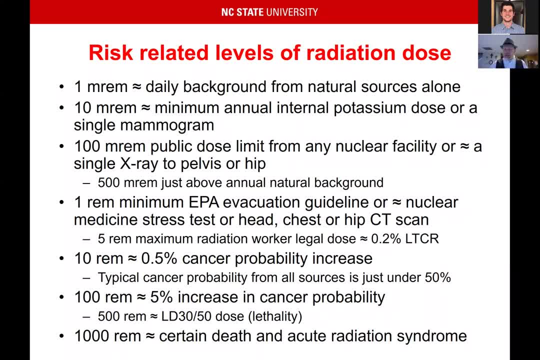 At 300 rem it would be 15%, And so they saw that with the atomic bomb survivors. And so really, what all of this stuff down here is is just extrapolating down to be conservative. So there is no measurement evidence other than well, if it's linear, it goes down there. 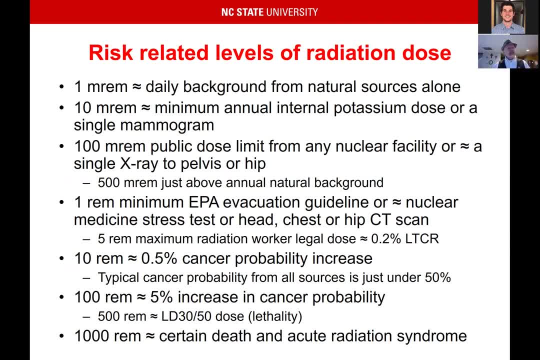 Now we know that that's not the case. That's actually not true in the sense that you can get these kinds. you can get doses bigger than that, just from background, And if you go to places where they do that, like Ramsar or Rann, that they get these kinds of doses per year just because there's a lot of thorium in the soil. 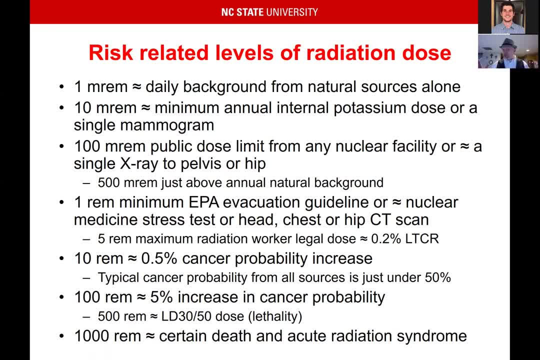 But those doses are protracted, That's averaged out over a year, whereas the atomic bomb survivors, they got it in a fraction of a second. And so there's a dose rate effectiveness factor that's just completely ignored in the linear no threshold. just to show again how conservative we are. 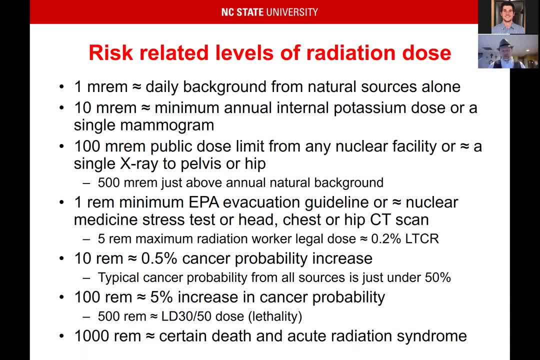 So we have a lot of radiation protection regulations which again will feed into radiophobia, And we'll talk about that later. So it's not until you get up to around 1000 rem that pretty much no medical treatment is going to help you. It's just like you got baked, like you were in a microwave for just too long and your body's immune system can't repair. 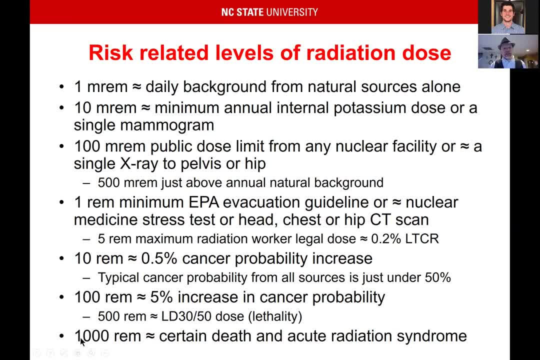 Down around 100 rem you start to be able to repair, And it's not until you get in the range of about 500 rem that around half the people that get that dose will die from acute radiation syndrome. So these are the big old, massive doses. This is where the threshold starts to be, where it looks like the body is able to repair itself If you let it. if you're not, 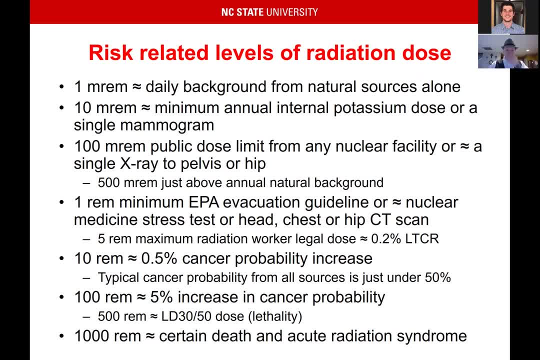 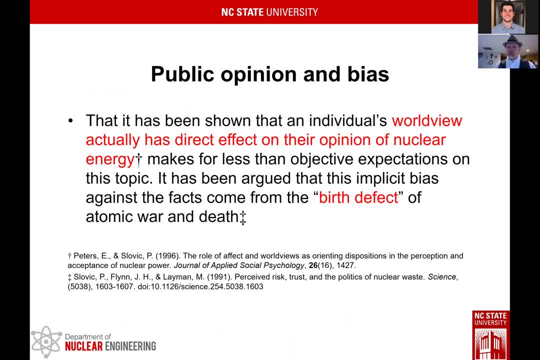 already. if you don't have a comorbidity, you'll be fine. That's what it looks like. So now let's talk about radiophobia. So what the literature is showing is that, for a particular worldview, that in and of itself will affect your opinion on nuclear energy. 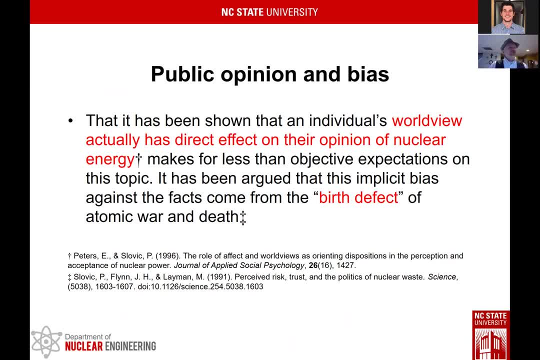 And so that might sound like a good idea. I don't know if that would sound normal or strange, But that would kind of like being saying: depending on what your religion is or your politics are, that's going to decide on whether you like electricity or not. 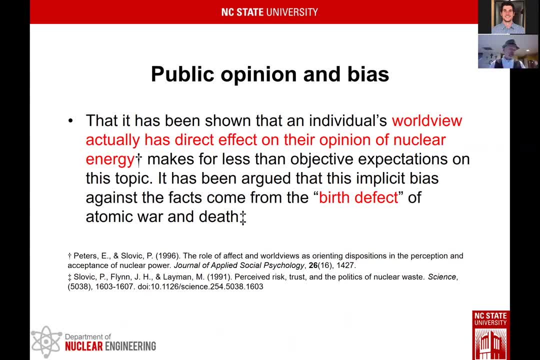 Right. So there are people that are like that, where for some religions they say we don't want electricity, And what the literature shows is the same applies with politics- that you can actually just have a bias on a technology simply due to your worldview. 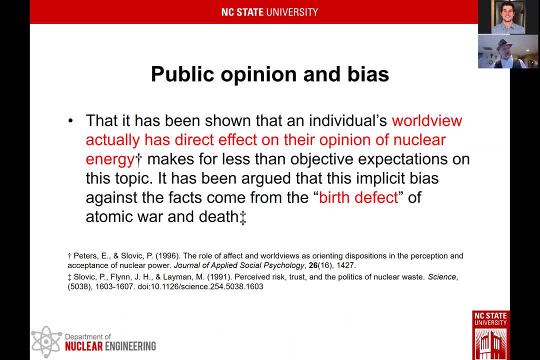 And it's also been attributed to the birth defect. Basically, nuclear technology largely exploded with the Manhattan Project. So we actually had it before the Manhattan Project, but because there was just so much money poured into the Manhattan Project, the knowledge just exploded with the atomic bomb. 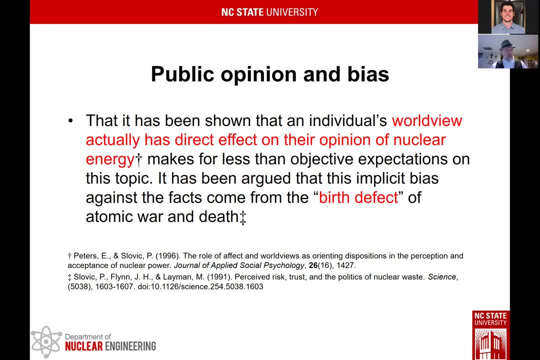 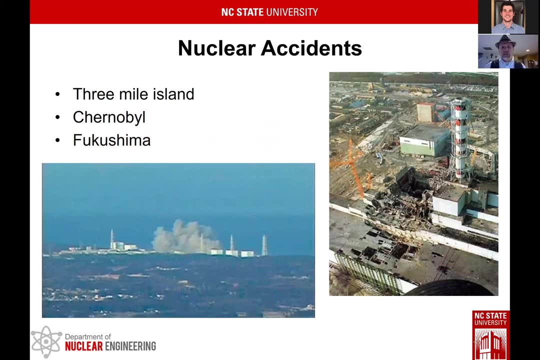 And so it's considered a birth defect that it really just exponentially increased in terms of the knowledge with the development of the nuclear weapons. So now let's talk about nuclear accidents. That's a really big issue When it comes to nuclear science and technology. that's on people's minds. So we'll go over really quickly Three Mile Island, Chernobyl and Fukushima. 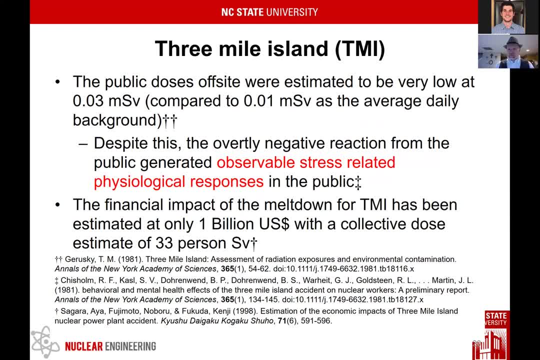 Three Mile Island was a terror event for many people and yet the dose was, for all intents and purposes, entirely negligible. So if you look at what actually people received, it was on the order of the average daily background, the total event right. 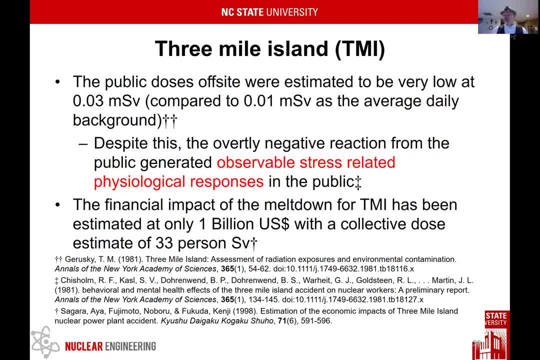 And yet people were terrified for having what, For all intents and purposes, was increasing your daily dose for less than a week, And yet it cost on the order of a billion dollars. it terrified people and it was a big fiasco in terms of being able to communicate this risk, because there really wasn't an infrastructure to be able to do that. 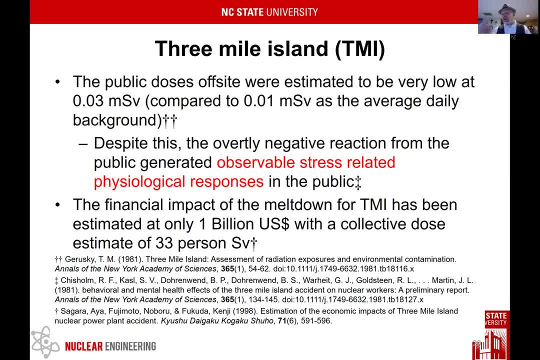 It was like who wants to talk? into the telephone, to the television, and whoever would talk, they would talk and they would give their opinion without it actually being vetted or having it backed by analysis. It was just their thought, Well, this could happen. 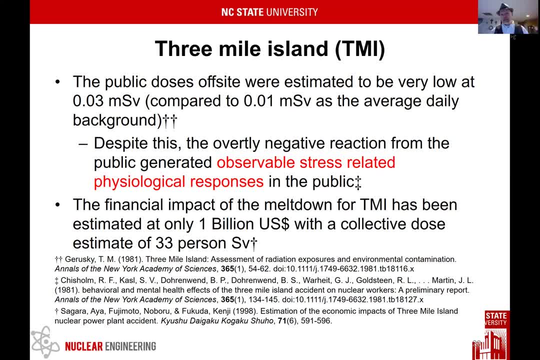 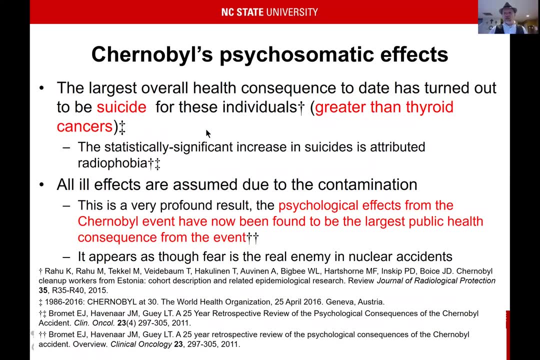 And so this could happen. then this is my opinion, And so it caused a big issue, even though it actually had a negligible effect in terms of offsite dose consequences. So the big one really was Chernobyl. So with Chernobyl, that was, I mean you almost could not have engineered something worse than that. 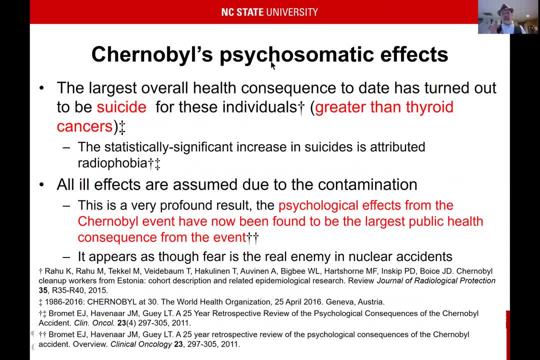 So the funny thing is that Chernobyl, even though it did cause a large number of deaths, Chernobyl was a big one. There were a number of deaths. There were on the order of about 30 people that died outright from acute radiation syndrome. 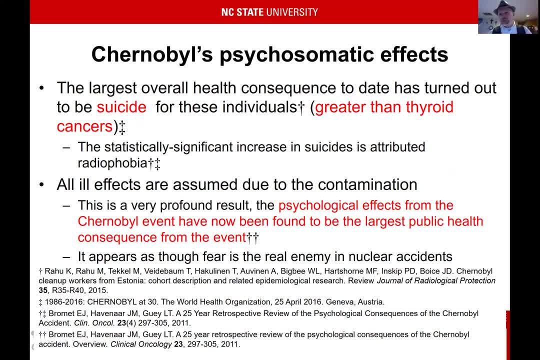 But now that it's been so long after the event that more people have died from psychological trauma than from actual radiogenic effects, So that's just crazy right. And what it comes down to is this thing called radiophobia. I mentioned it before. 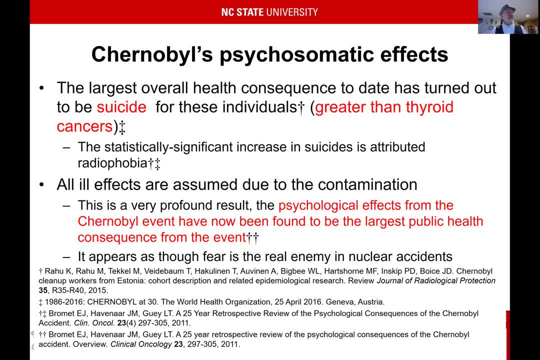 Now, radiophobia when it comes to these kinds of effects is kind of like if somebody said to you that you have been cursed, You now had a curse, Then if you believe that, then that can cause stress And if you have stress, that will reduce your immune system. 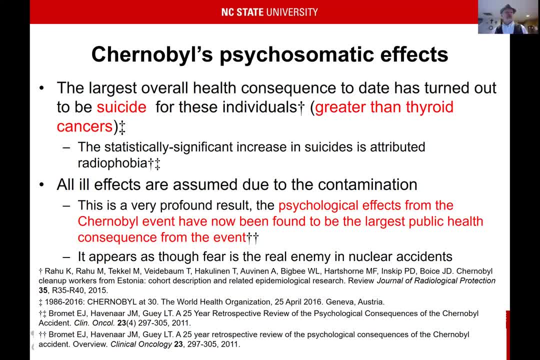 And if it reduces your immune system, you're more likely to get sick. And if the curse told you you were going to get sick and you get sick, it's like a self-fulfilling prophecy. And so that's what happened to these people in Chernobyl. 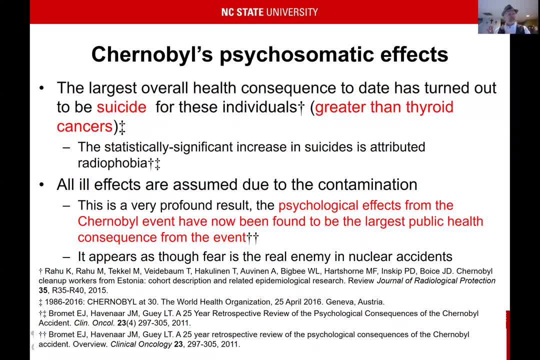 Literally, they become like a radiation person. They get a stigma and they attribute any bad thing in their life to Chernobyl. And it's just this self-reinforcing condemnation that they have no hope, And so the suicides have now increased. 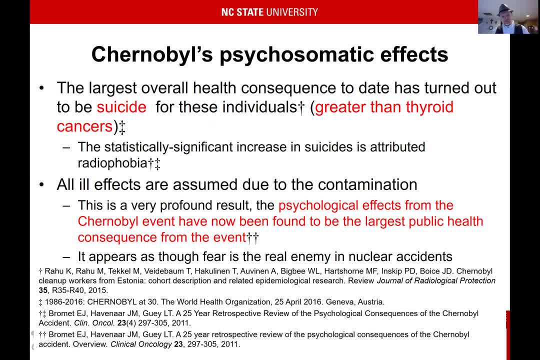 The suicides have now increased, above and beyond the radiogenic deaths, which was an entirely unexpected result. That was just crazy. So the literature now shows that the psychological effects are worse than the radiogenic effects. Can you imagine that It's just because you're so terrified that that causes more health problems than the actual, even though it was the worst case that you could imagine? 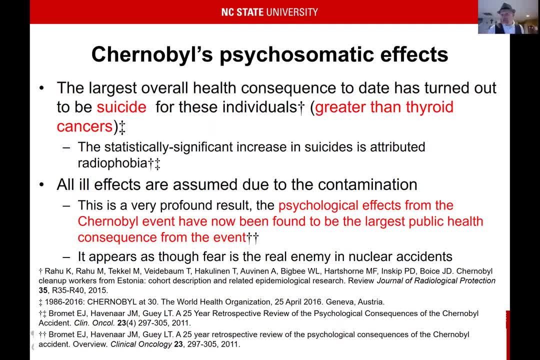 You really almost couldn't make something worse than that, unless you hit it with an atomic bomb. You really couldn't design it to be too much worse than that, And that was, That was the Russian design. So now let's look at what happened from Fukushima. 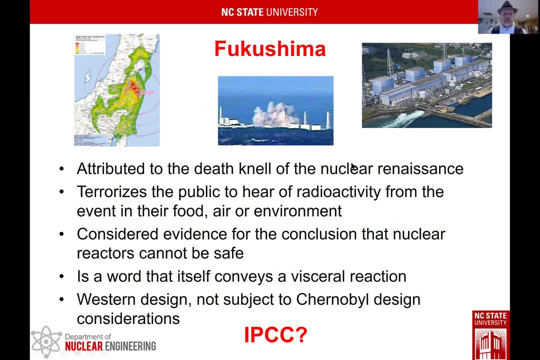 So Fukushima was attributed to the entire death knell of the Renaissance. So, even though nuclear looked like it was coming back, this was a Western design. This was a design that came out of the West with all of our safety criteria. How is this even possible if this managed that? 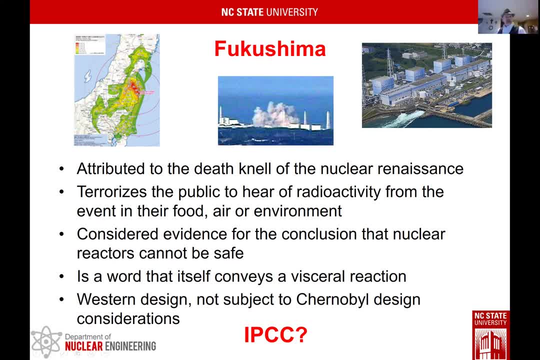 So I bring down here the International Panel on Climate Change. I'm going to make a few assumptions on world views of our students. I'm going to assume all of our students believe the International Panel on Climate Change. If you do disagree, then we can talk about it at the end. 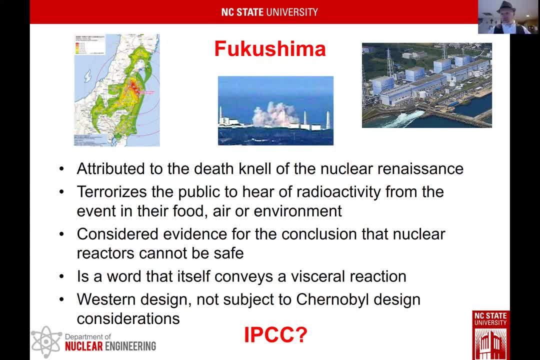 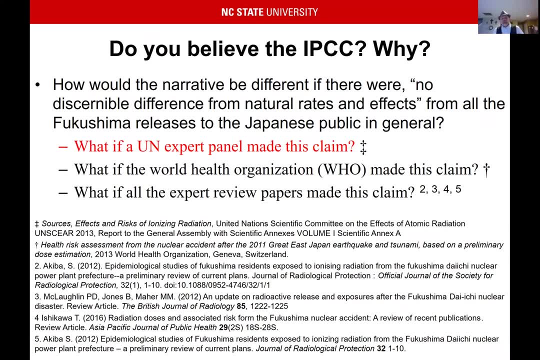 But I'm just going to make that assumption for the purpose of this presentation And I'm going to do some other assumptions And you can challenge me later and that's fine. So if you believe the International Panel on Climate Change, I would ask you why. 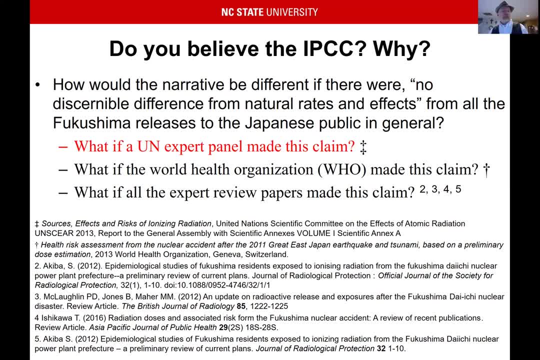 I'm assuming that you do And you're going to say: well, the United Nations put together a panel of experts from around the world And they looked at the evidence And they all agreed. And then all kinds of other professional societies agreed. 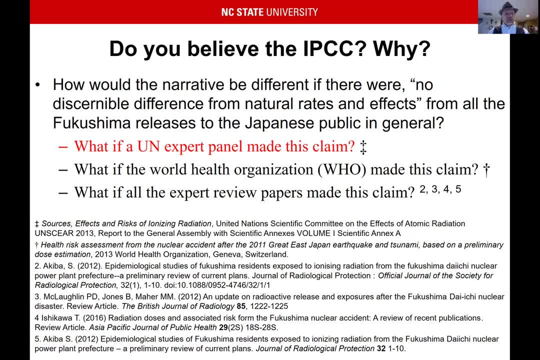 And all of these other climate scientists agree. Even the World Health Organization agreed and so forth, And there's only a handful of climate scientists here and there that would disagree. You might say: well, as long as there's one or two of these climate scientists that agree with me that there is no climate change, I'm not going to believe it. 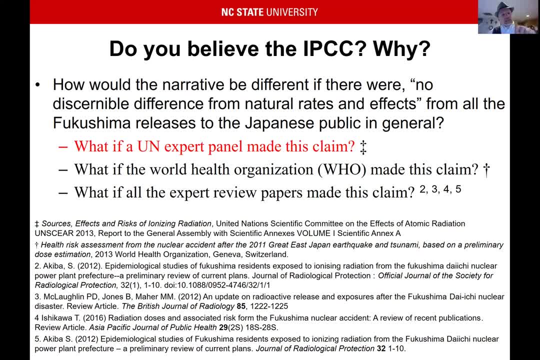 I mean, there are people that are like that, But the point that I'm making here is that what if- and this is a hypothetical- what if? the United Nations put together an international panel of experts to look at the health effects from Fukushima? 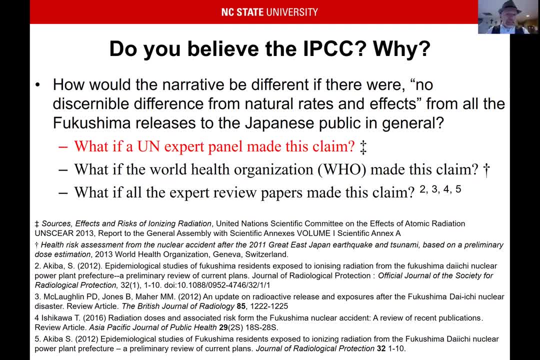 And then that panel then all concluded in consensus that the dose was too low to the general public to cause a single measurable medical effect from the entire release of Fukushima. So you would think that would change the entire narrative, that people's attitudes would completely reverse if something like that happened. 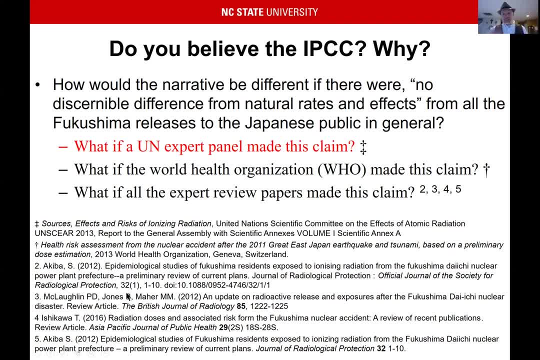 Well, truth is down in these references. that's exactly what happened. The doses to the public were too low for a measurable medical effect- Remember, if it's in the range of 10 rem, you can't see it- And so the doses were even substantially lower than that, down in the range of what you already get from some places in nature. 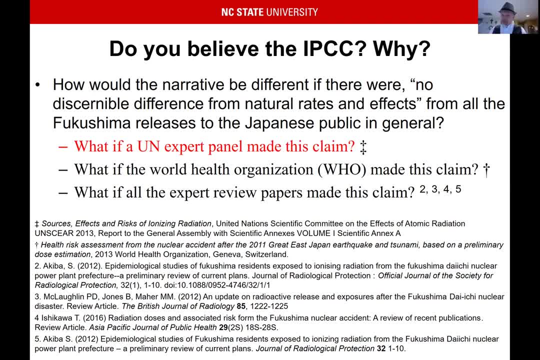 And so the World Health Organization said this, All of the professional societies said this. In fact, I've never seen a credible nuclear engineer or nuclear scientist that disagreed with this. What I have seen is that they say: well, nuclear terrifies people so much that we need to just go away from it because there's too much public opposition. 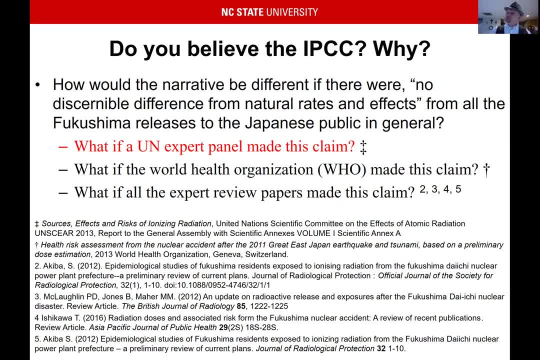 It's actually a good point. And then they also say the same thing applies with Yucca Mountain. The public are opposed to it because they're so terrified of it. They were not going to be able to have a place to put the waste again because of radiophobia. 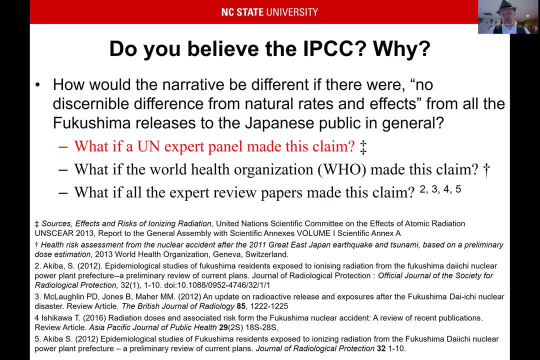 And you know you can't quite argue with that, because it's true. Radiophobia actually causes this to not even be seen, even though this has been seen, this has been done, And they've even done multiple studies after this and reinforced it. 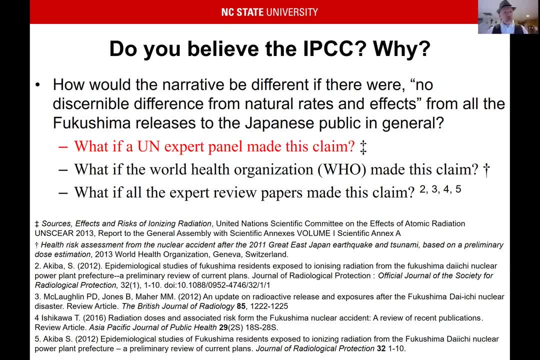 No measurable medical effects from the entire Fukushima release. All of it was too low for the general public And that's just in Japan. That doesn't count for people over here or people anywhere, That's just for the people in Japan. It was below measurable levels. 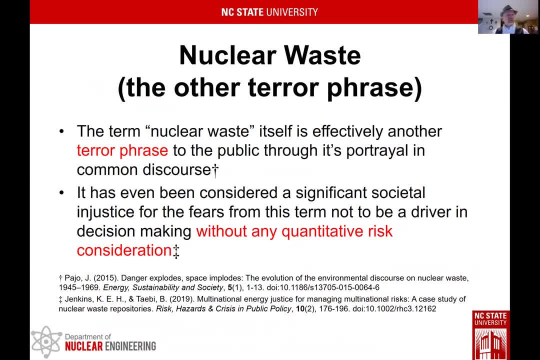 Another example is nuclear waste. I kind of mentioned that. That's what some of the experts will point out is that people are terrified of it. In fact it's been shown in the literature that it's almost like a terror phrase, That if you say nuclear waste, people are thinking that there are these horrific accidents that are just going to kill everybody. and yet nothing's ever happened. 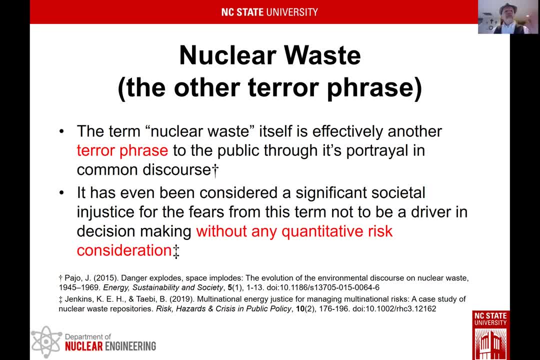 There has been no technical analysis that's been done. even though it's used in the literature as a proof of why nuclear energy is bad, Even though there is no quantitative risk analysis that's associated with it, it's just used as like a proof, kind of like a default. 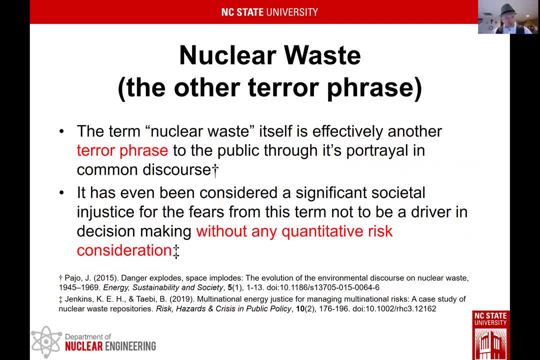 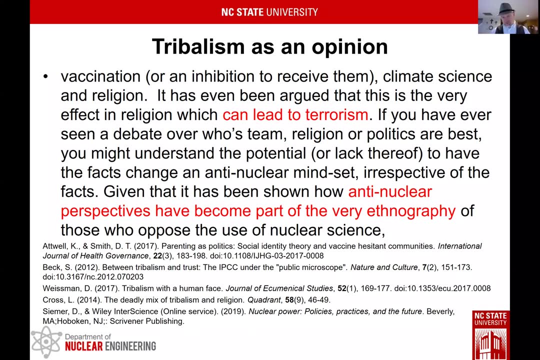 It's this ethos that's built in, This systematic belief that just the word is proof alone. and that's it. Now the literature says that this is actually a form of tribalism. Tribalism is something, apparently, that's very natural to us. 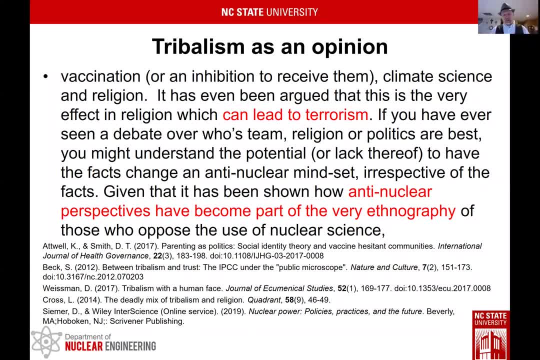 It came from coming out of a hunter-gatherer evolution such that you will automatically- or you naturally will- be biased to think that whatever your tribe is, it's going to kill you. Whatever your tribe is, wherever you were born, your tribe is good and then the other tribe is evil. 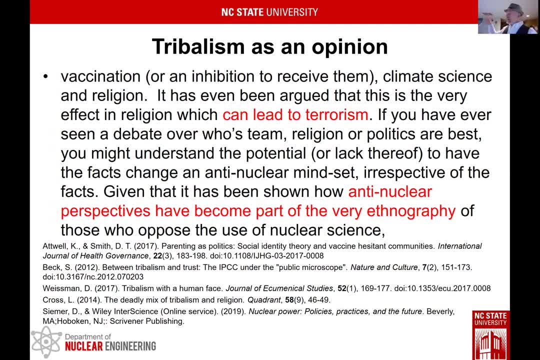 And then when your tribe does something bad, it's in spite of the fact that you're good, And when the other tribe does something good, it's in spite of the fact that they're bad. And that was a survival mechanism to help each tribe support itself and keep itself sustained. 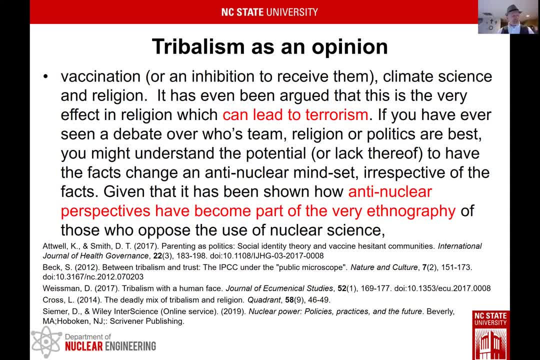 So you can see what's wrong with it. right, Every tribe is doing that. right, And it doesn't just apply to technology. There's this natural bias to think that the school that you live by is the best school, or the soda, or the car manufacturer, or whatever. 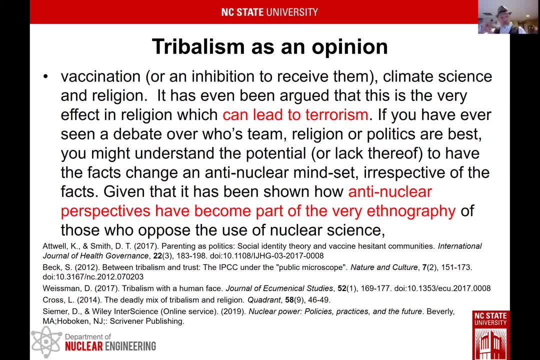 You have this tribalism, where the narrative is collective and that you have to adopt that narrative if you're going to be a part of that tribe. So that's literally become part of the ethnography of our nation. That's what this literature down here shows, which means that it's assumed to be true without proof. 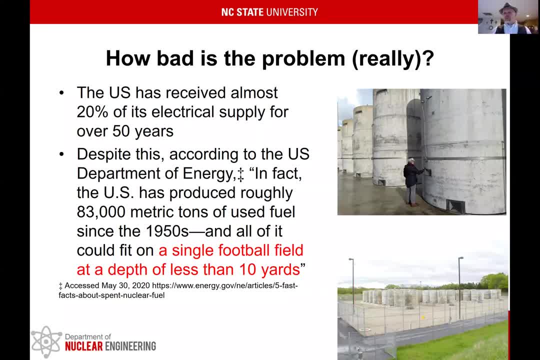 Right. So when it comes to nuclear waste, how bad is the problem? So if you think about this, since the 1970s around 20% of all of our electricity has come from nuclear. That's a lot. Since the 1970s, 20% of all of our electricity from nuclear- and it would not fill a single football field above 10 yards. 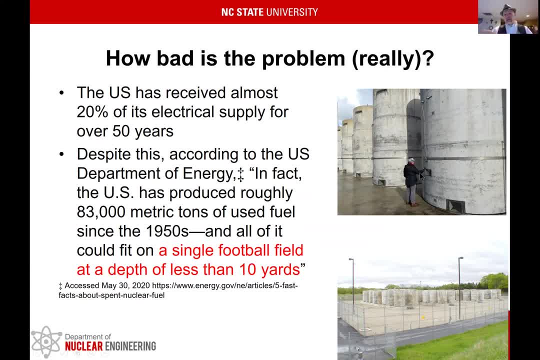 Three meters high. If you put these things on their side and rolled them into a football field, all that's out there would not even fill a single field. And that's just because of the energy density. The energy density of nuclear. the amount of energy that you get per reaction is, you know, hundreds of millions, at times about 200 million electron volts per fission. 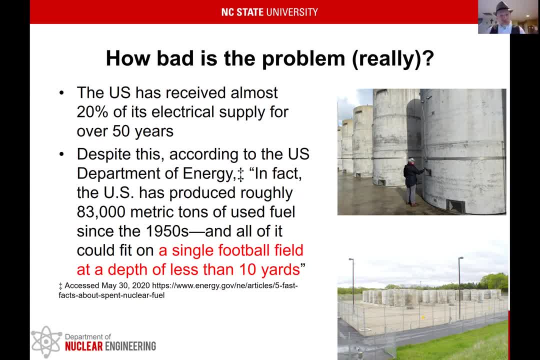 Whereas with chemistry you might get, say, one electron volt per atom in a chemical reaction. So it's just a huge energy density difference when you're making heat with nuclear as opposed to burning fossil fuels. So it's really not as bad as people think, especially since there haven't been any accidents with this material. 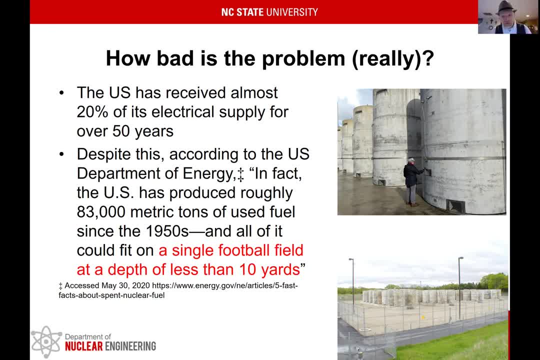 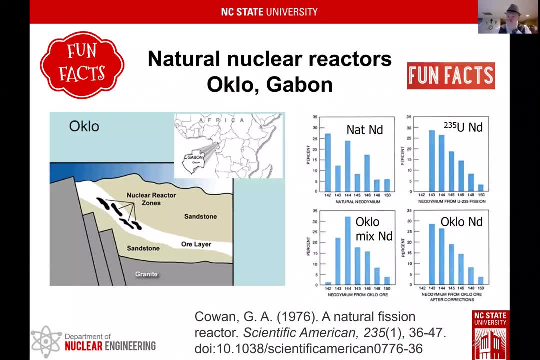 And it's easy to control and handle and it's a very small amount. So the smaller it is, the easier and more cost effective it can be. So I'm going to do a little bit of a rabbit's trail, a very cool rabbit's trail. 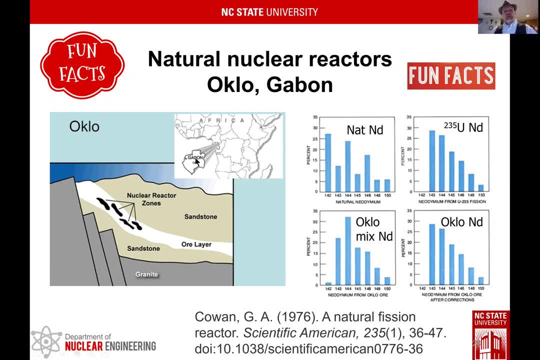 And I'm going to talk about this place in Africa, Gabon. There's a uranium mine there And in that uranium mine they found that all of the natural isotopes had some perturbations to them, Very strange perturbations. 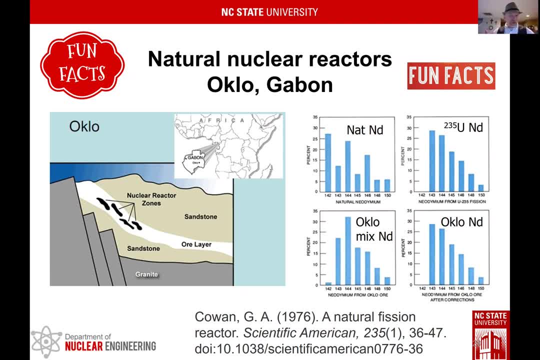 Because it started with recognizing that the fissile component of the uranium, uranium-235, was less than it was anywhere else on Earth as far as we've ever measured. And they found out the reason why is because that fissile uranium-235, it's got a shorter half-life than the fissionable uranium-238.. 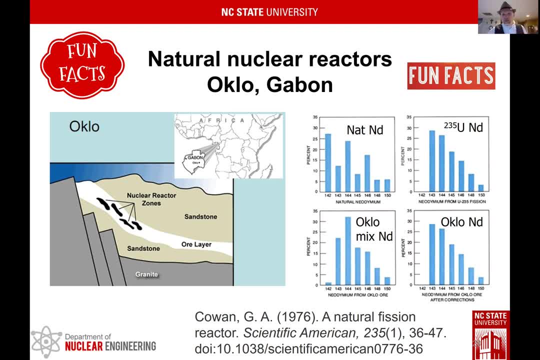 Which means if you go backwards in time a few billion years, the uranium-235, which is decaying, faster forward, it enriches faster going backwards. So back a few billion years after the formation of the Earth, the uranium that was naturally in the Earth would have been around the same enrichment that we have in commercial nuclear reactors now. 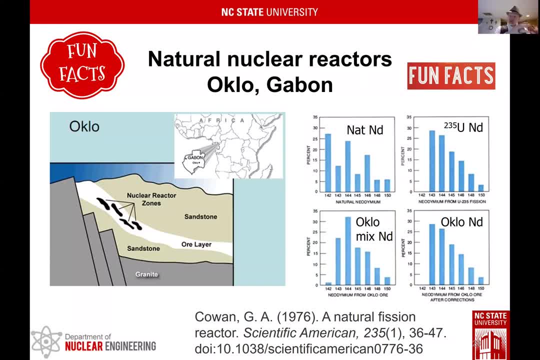 And what that means then is that if you had geology that concentrated it in a geological formation and you got some water in there, it would go critical, And that's what happened here. And so if you look at the natural neodymium that we get elsewhere where there isn't any uranium, and you look at what you have for the oaklo, 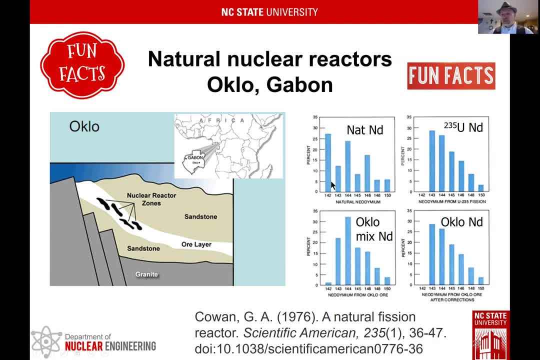 it turns out in oaklo it's a linear superposition of the natural neodymium isotopic distribution And that from the fission, the decay chain isotopes from uranium-235 fission, So that the neodymium addition to the oaklo mix that's required to get what's measured is a fission distribution. 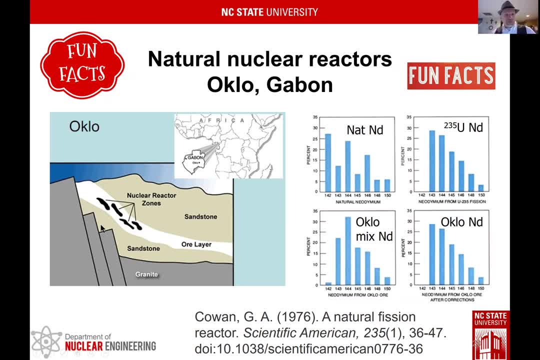 which shows that the uranium actually did fission. And what's significant about it is that the nuclear waste stayed in the ground. It didn't move. So this is an empirical demonstration that you can dispose of nuclear waste. You can dispose of nuclear waste in a geological formation and let it sit there until it just becomes dirt. 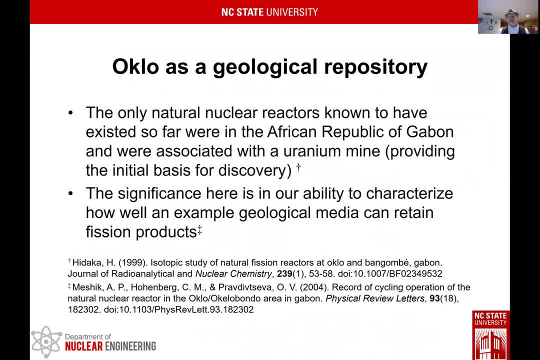 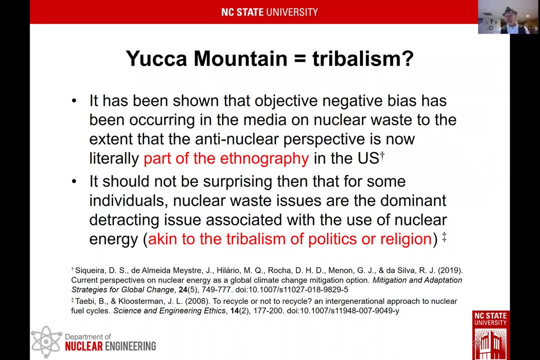 Just a different kind of dirt. Oh, and I already talked about this. Okay, All right. So Yucca Mountain literature also shows that it's become tribalistic, That you just need to mention the word and it's all arms go up and say, yeah, that's proof you shouldn't do nuclear. 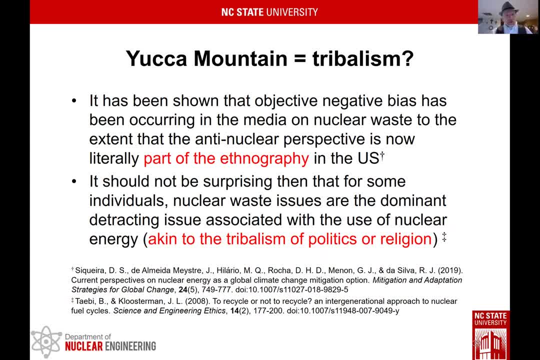 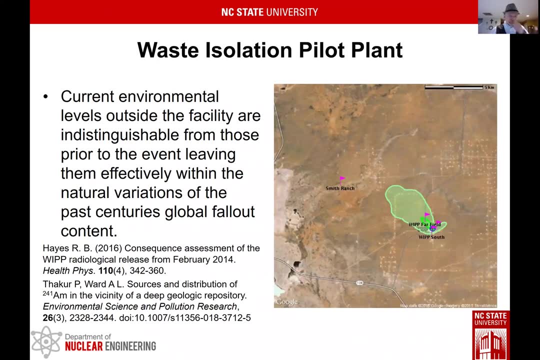 It's like it's an assumed truth with no proof. So it's an ethnography. It's part of the narrative of the tribe, which is similar to politics and religion. That's considered also a natural predisposition that we as humans will naturally default to some kind of a collective tribal narrative. 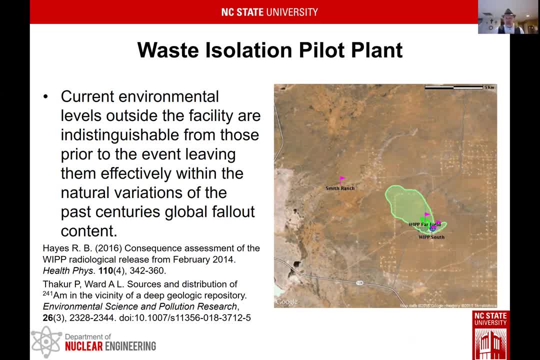 So here is actually an example of a geological repository where there actually was a release. This is again a worst case scenario: A drum deflagrated and it basically dumped all of this stuff into the repository and the repository safety features leaked. 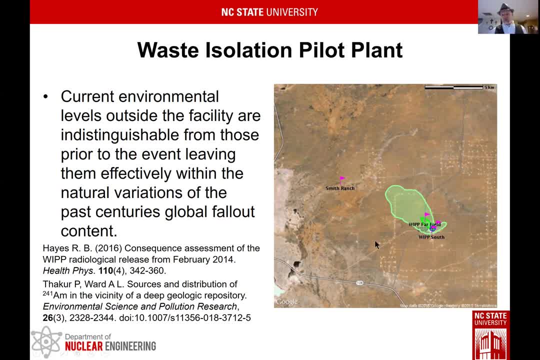 Funny thing is is that, Even though this terrified people, people were thinking of moving literally because this was the plume. This was a verified, validated plume, And you can see these little purple flags. That's where we actually measured it and we were able to demonstrate: yep, that's what it was. 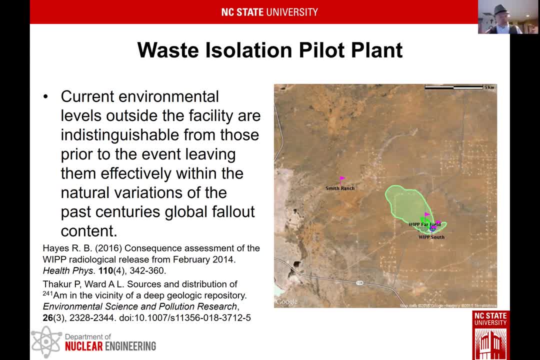 The model was normalized to the measurements and they agreed quite well, giving us confidence that we did understand it and that we did correctly characterize it, Even though we were able to measure. this turns out that the actual plume here was on the order of it was comparable to the actual plume. 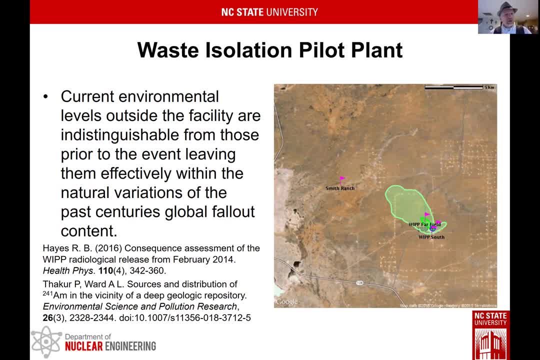 It was comparable to the actual atmospheric weapons fallout from the prior century. So let me say that again, We have atmospheric weapons fallout all around the Earth because in the past century the nuclear weapons countries have been doing atmospheric weapons tests out in the Pacific or out in other places around the globe. 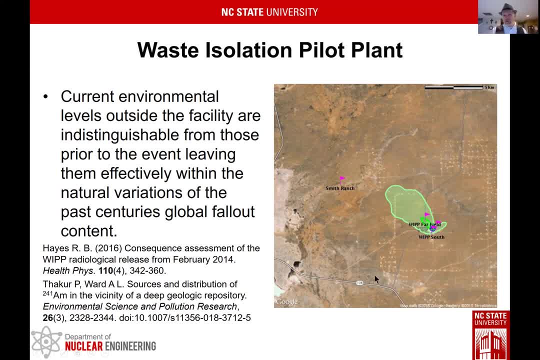 And so the fallouts all around the world, including americium, which is what this was, So the actual americium that was deposited out here in public land, It just around doubled. what was there doubled? what was there prior to the building of that facility? 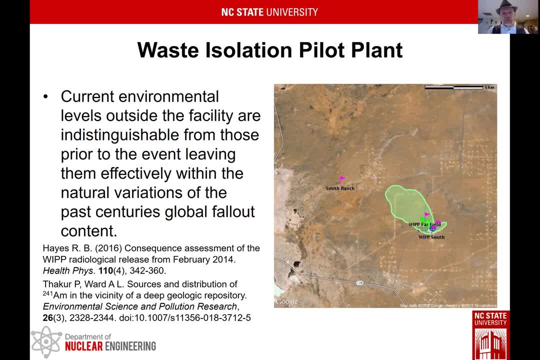 So it was, in a rather literal sense, trivial, because you can naturally get concentrations of this stuff, the fallout, based on its solubility and how it transports with water. And so, even though it was a trivial release, it really was a big deal in the sense that it was not planned and it was not controlled. 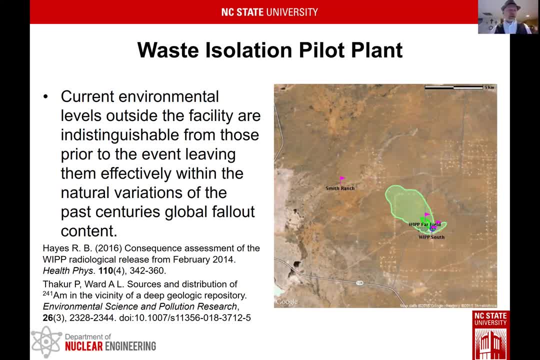 And when that happens, that means that if you don't do anything bad, pretty much just getting lucky because you weren't controlling it and it wasn't planned. So how do you know? it couldn't have been worse. In a sense, it was kind of like Chernobyl. 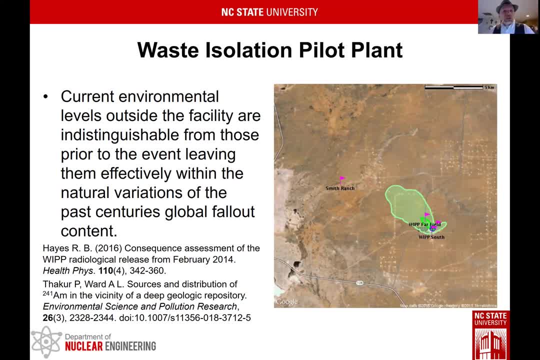 It was about the worst that you could possibly get. It was like having a dirty bomb. I would say it was having a dirty bomb go off in your repository. It's pretty hard to imagine something worse than that, But the point is is that the safety features work like they did at Fukushima, which is why the actual release was trivial. 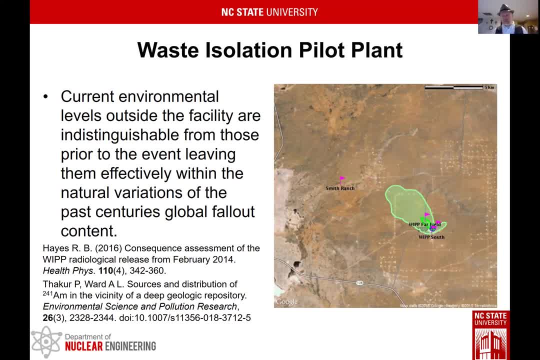 Because it was designed for this work. Right, It's the worst case. That's how we do it in nuclear. We just assume the worst thing is going to happen And we say, all right, if the worst thing happens, let's design this so that people at the fence are going to be safe. 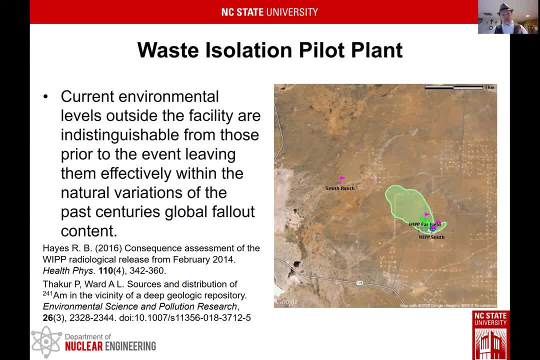 And even though that worked and it was supposed to be that way, it doesn't mean people weren't terrified, And they were. They were terrified Because, remember, the EPA will issue evacuation guidelines telling you to leave your house if you're going to get a dose every year comparable to getting a chest X-ray. 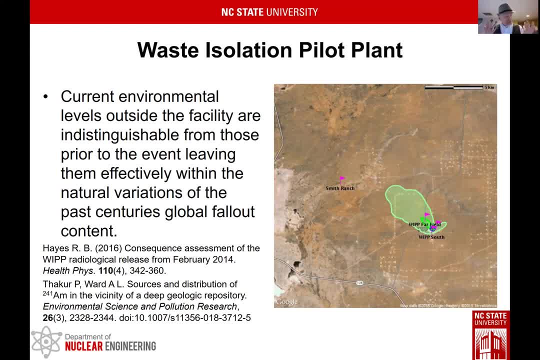 So that might not make a lot of sense that that's the way that our regulations are. They're just that conservative to protect the weakest in the society. Because, if you're getting again, 10 rem is around, where we're just able to see measurable effects in children. 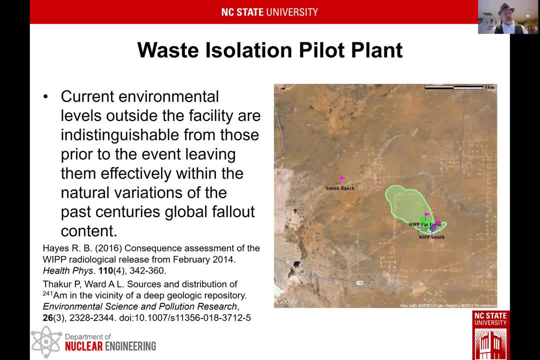 We don't see those in adults, But in children. for children that have gone through radiotherapy, that's right around the threshold. So if you're getting one rem from the earth right, you could be getting another nine rem from somewhere else. 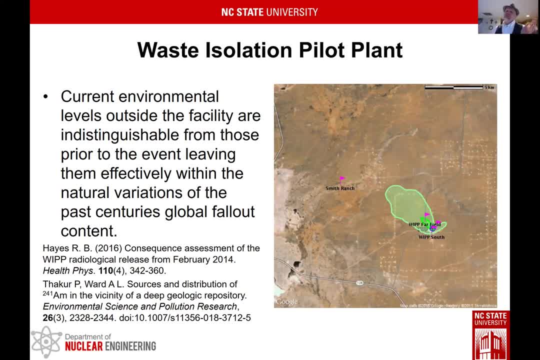 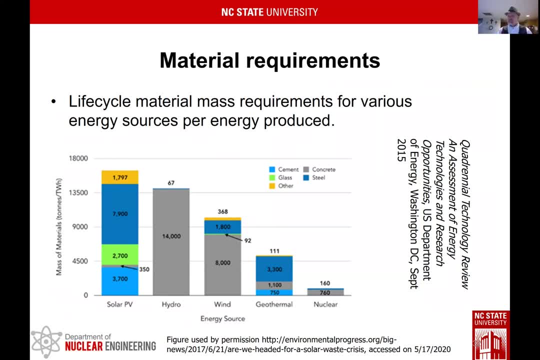 Even though that doesn't take the dose rate effectiveness factor into consideration. But that's just how conservative those things are. So now let's talk about some real engineering. So let's not look at the radiological risk, but the engineering risk management issues. 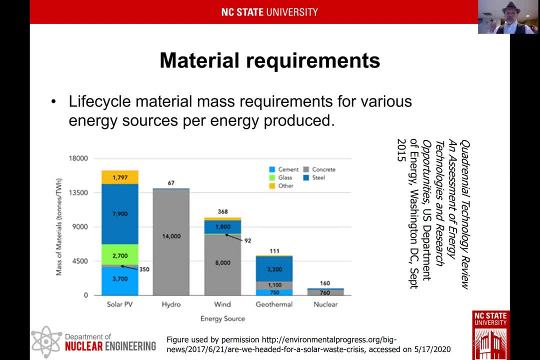 And so this came from the Department of Energy, And it comes down to how much material is required to generate a gigawatt, or in this case a terawatt, Because with nuclear it has a huge energy density, So the amount of material that's required, 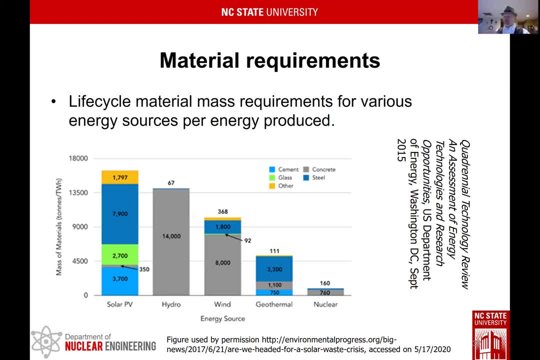 So the amount of material that's required to do that. Remember all that material, most of it's being manufactured- the concrete and the steel- Most of that's being manufactured with energy, from fossil fuels, from coal and natural gas, And so you don't want to have a lot of that. 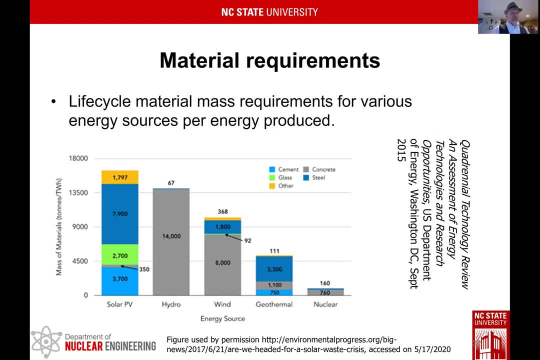 You want to get a lot of energy with only having to generate a little bit of greenhouse gases, And when you make the actual installations, that's going to require materials which requires energy. And you can see, when it comes to what are considered the traditional renewables, nuclear has the lowest. 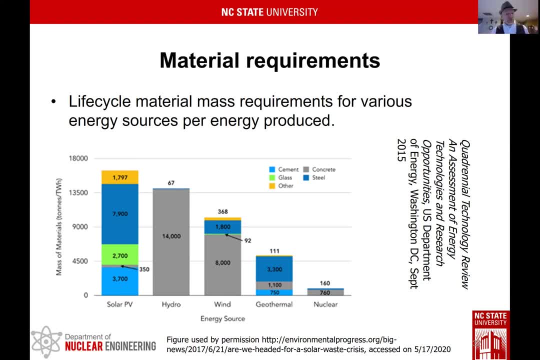 Because it just has so much energy over such a long period of time. it doesn't need to be replaced as often as, say, solar panels or something like that. And solar panels, they have a much lower energy density. They don't give you as much energy for materials that you have. 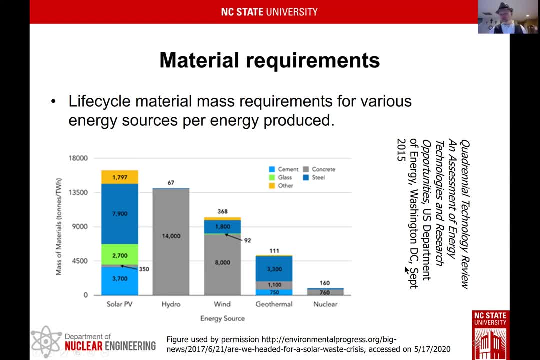 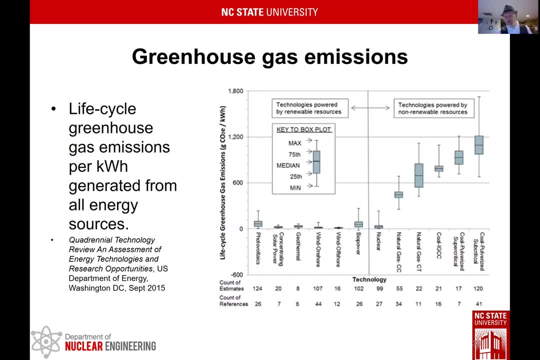 And so nuclear is the lowest. So from that perspective it's entirely green relative to this metric. Another metric is greenhouse gas emissions, So it's not just how much materials are required to generate a gigawatt, But how much greenhouse gas is emitted per gigawatt. 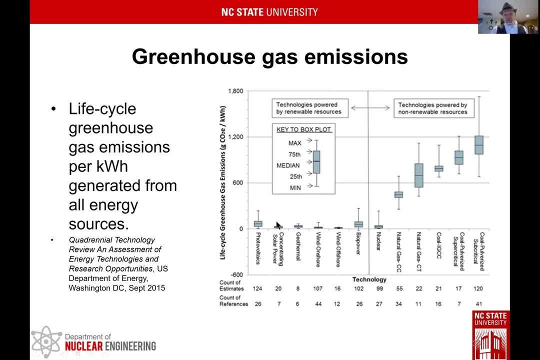 And when you look at the traditional renewables over here you can see nuclear is as good or better than some of them, And it's as good as most of them in terms of greenhouse gas emissions, because it doesn't release greenhouse gas emissions Like the rest. right, if you have wind, you've got to drive a truck in there to get a person to go up and do maintenance. 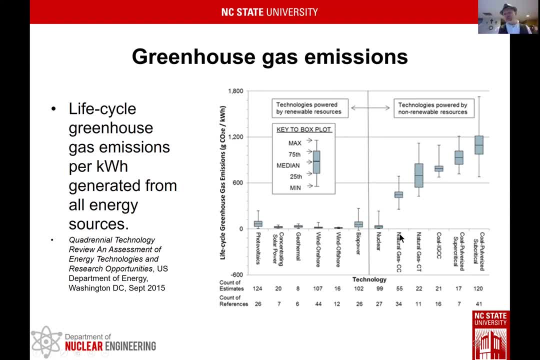 And that truck releases some greenhouse gases, And you have trucks at a nuclear power plant or anywhere else, And so that's a good metric, And so that's why these are so low. They're not zero, because there are other facilities or other infrastructure that does still use greenhouse gas. 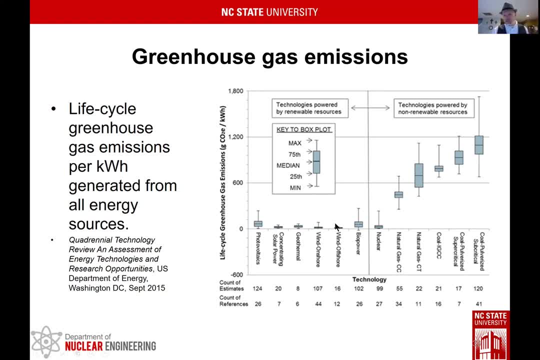 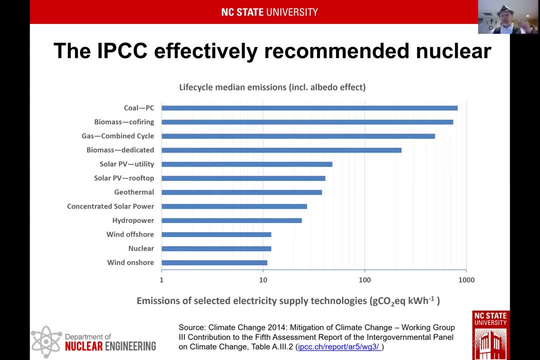 Mainly it's gasoline, stuff like that, But you can see that it's extremely low compared to the others. So even the International Panel on Climate Change, when they issued their recommendation saying we need to control climate change, they actually called out nuclear. 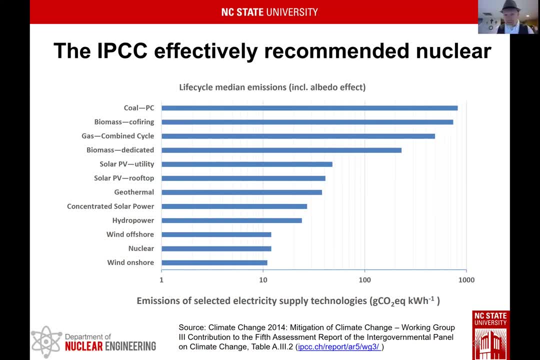 They actually said: you need to do nuclear. You're going to have a real hard time making these goals if you wipe out nuclear, which a lot of countries have done. They said, well, we're going to do it without nuclear, We're so smart. 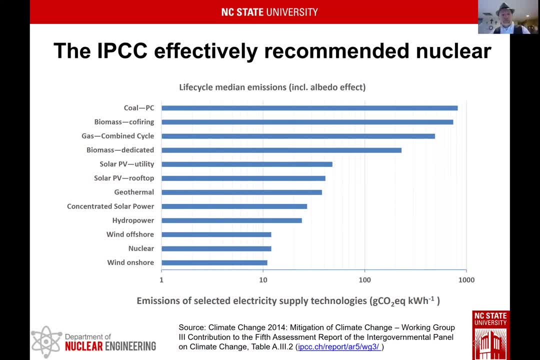 We're so great We're going to do it without nuclear And God bless them. I hope they do it. But operationally and effectively it's going to be very difficult because of such a massive amount of electricity that you can generate baseload and it doesn't release greenhouse gases. 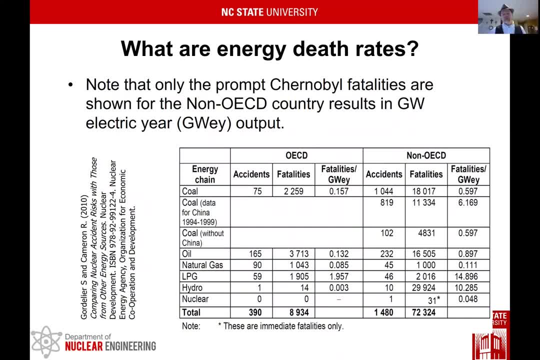 So another thing that I would think should resonate with people is: what is the death rate, What is the actual death rate? And if you go to the non-developed countries versus the developed countries, what is the actual death rate? If you're looking at- and these have been tabulated by the OECD- nuclear looks incredibly impressive in terms of the number of people that die per gigawatt electric year that's generated. 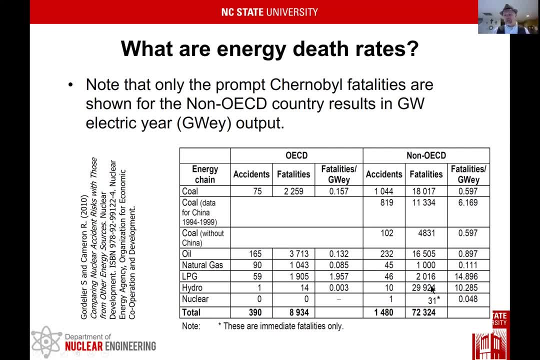 Now the numbers over here are for Ukraine, which is not an OECD country, and these were only from the outright deaths. The actual number of cancers afterwards are in the thousands. But those are the people that died from the acute radiation syndrome And you can see that in the US hydro is really good right. 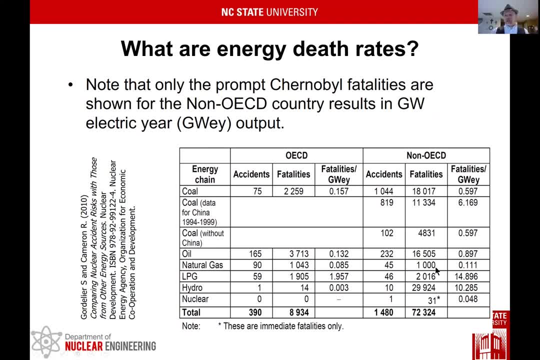 Unless you're falling off the dam, things are pretty safe, Although in the non-OECD countries you know, sometimes they use an earthen dam and if that breaks you're going to kill a lot of people. But the point with this is that in principle you would think it should be just as bad to die from- you know- natural gas as from coal, as from hydro or from nuclear, that a death from nuclear isn't any worse or any better than a death from anything else. 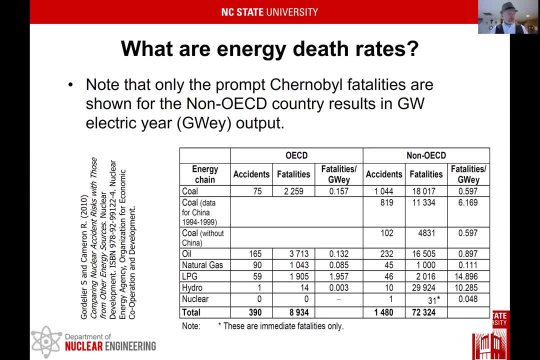 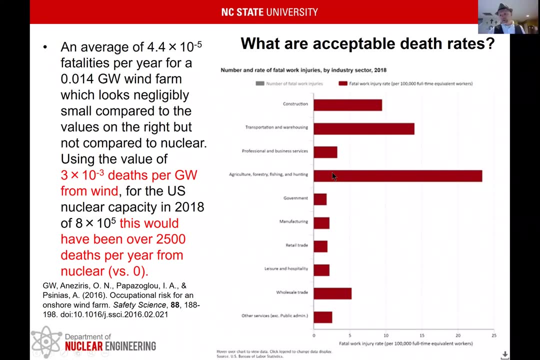 But that's where that ethnography comes in. The ethnography says that a death from cancer from nuclear is worse than a death from a trip or fall if it's from, say, solar or wind, And here's an example of that. So these are the safety rates that you get from various industries, from construction, transportation. 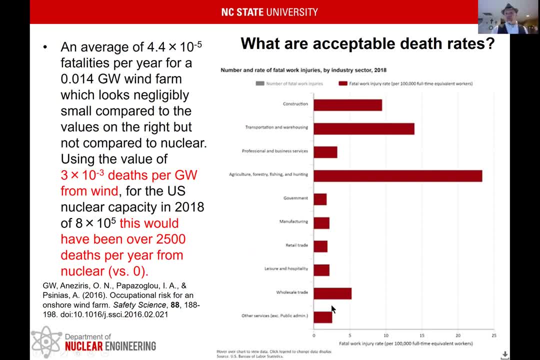 You can see, agriculture that's the worst, right Farm accidents, And so these are the number of fatalities and work injuries that you get from a standard assortment of industries that we have Now, in order to make a comparison for nuclear, I pulled out this paper of the fatality rate at a wind farm in Greece. 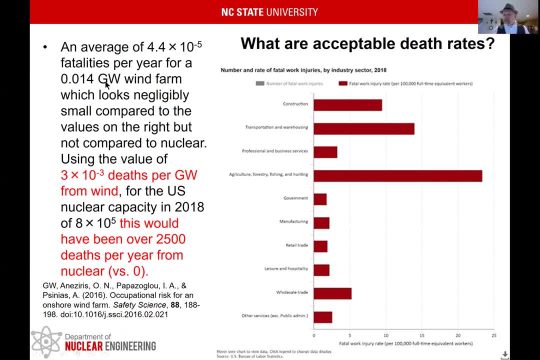 So it's a small one, It's only 14 megawatts, But every now and again a person will fall from one of the turbines or something like that will happen, and then they will die. So that gave three times 10 to the minus three deaths per gigawatt. 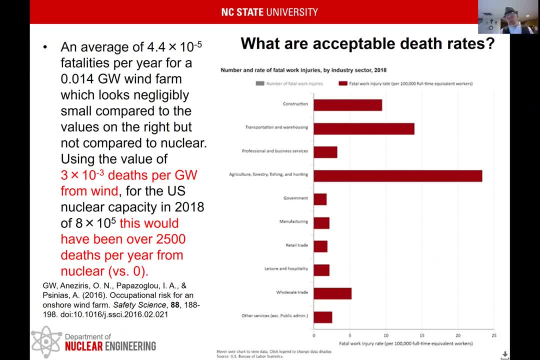 Now that sounds really good and it could be a lot worse. I mean, still, any one death is unacceptable, but the point is that's a really low number. So if that's what it is per gigawatt, if you compare that to nuclear, which generates substantially more, many, many gigawatts- instead of 14 megawatts we generate many tens of gigawatts. 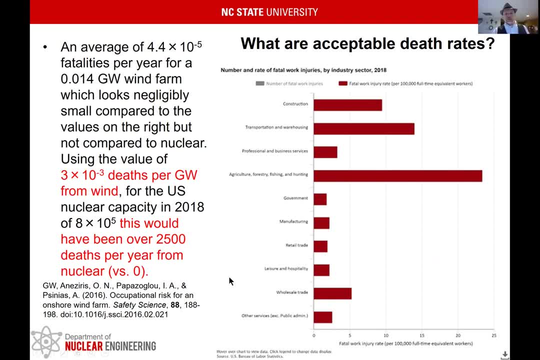 If you scale that up, that would have been at this death rate for the nuclear in 2018, that would have required 2,500 deaths And we had zero. And so, again this comes back to the ethnography. 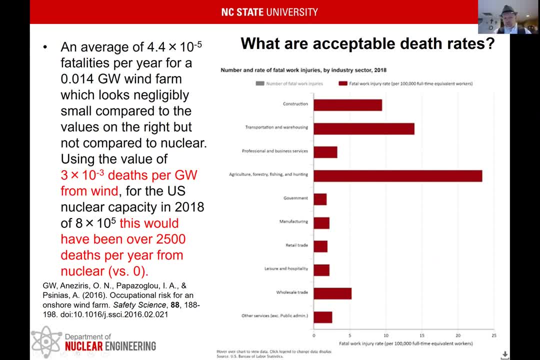 Well, dying from wind is okay, but dying from nuclear is not. Dying from wind is not, Dying from nuclear is bad. That's where that ethnography comes in, where you don't have to have a rationalization. It's just an accepted truth, without a challenge. 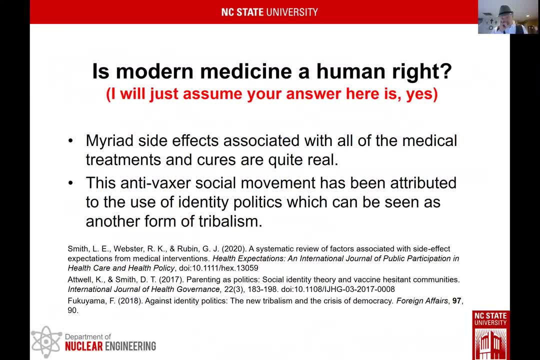 And so this is just a good example of that. So now, as I come to the end, I'm at the end of my 45 minutes, so I'm going to make another assumption. I'm just going to assume, for the sake of discussion here, that you agree that modern medicine should be considered a human right. 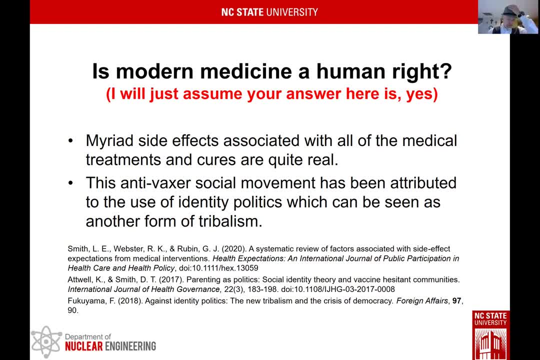 But now I'm going to put on my engineer hat. So I've been wearing my health physics hat, I'm going to wear my engineer hat. I'm going to point something out here. So as good as that statement is, it's worth recognizing that without technology, you don't have medicine, right? 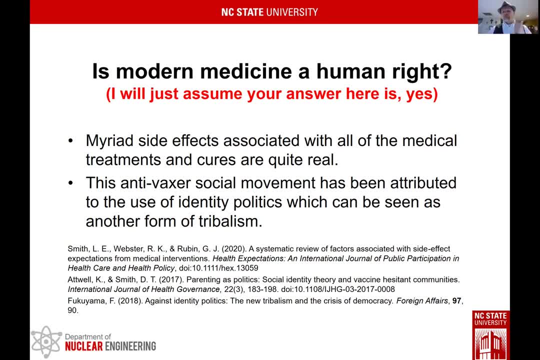 Without. if a person doesn't have clothing, they're probably not going to care about medicine. If they don't have housing, I don't know how much they're going to worry about medicine If they don't have clean water, if they don't have heating in the winter or cooling in the summer, maybe medicine? 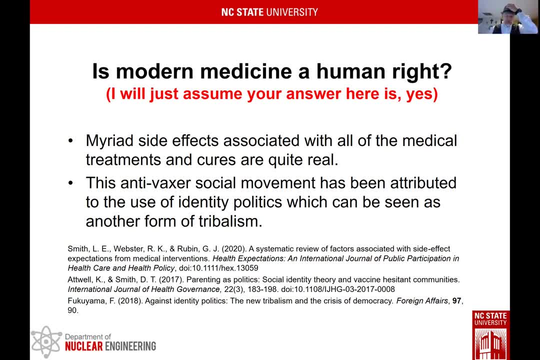 isn't quite so important. But if they don't have transportation, they can't even get there. And so all of these things that I just mentioned right to be able to have clean water, to be able to have food, to be able to have heating, clothing, housing, all of that requires electricity. 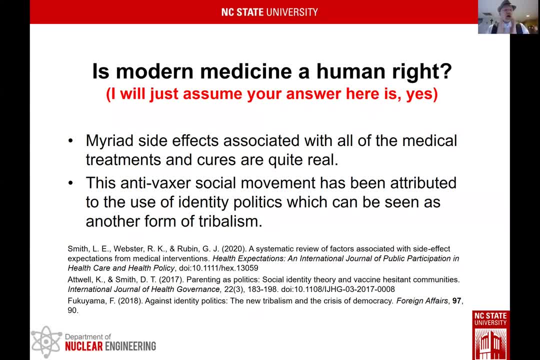 And so electricity, fundamentally, is really what supports our society in terms of maintaining these systems, of systems that give us not just our standard of living but our ability to live, And electricity is not even considered a human right. But if it is, then where is it going to come from? 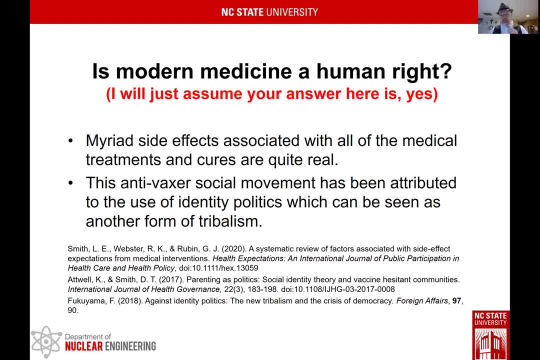 Because all of this is predicated on the idea- just think about Texas right now on having electricity- And as long as we allow a narrative that is strictly not based on science or is strictly not based on any kind of objective analysis other than 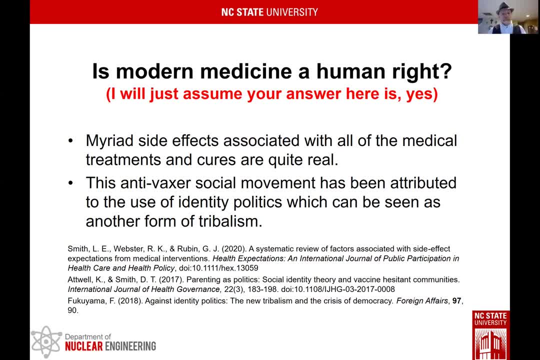 this is what I want to believe, and so I don't need to prove it. we're going to have those difficulties that the anti-nuclear nuclear engineers point out, And that's that. the public just doesn't want it. The public does not want nuclear. 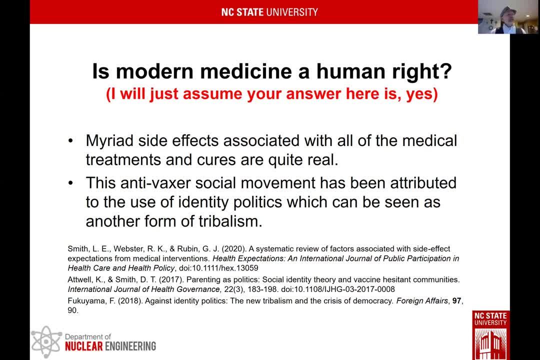 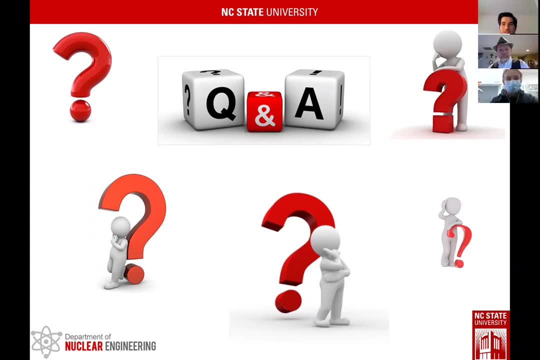 They're afraid of it, They think it's evil, They think it's bad, They think that nuclear waste is a terror phrase. And that leaves us at the end of my presentation. Thank you very much. That was fantastic. We have three questions ready to go. 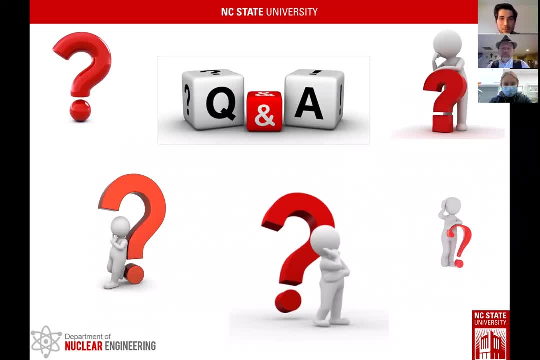 So I'll go ahead and ask One's from an anonymous attendee. But their question is: what were some of the uses of nuclear energy before the Manhattan Project? Oh, that's a fun one Great question, All right. So before the Manhattan Project it was discovered there was a really famous project that was done that the word cancer. actually comes from one of the. I don't remember if it was Greek or Latin. I think it might have been Greek, might have been Latin, But it comes from the word. that means crab, And that's the way the cancer looked at. it appeared on the surface of the body. 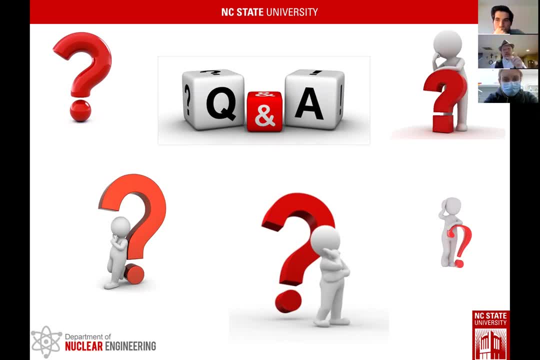 And when radium was first discovered, there was a physician that actually decided to try this on a cancer. A person had this massive tumor on their face And he started applying radium exposure for a long period of time And the cancer went away. 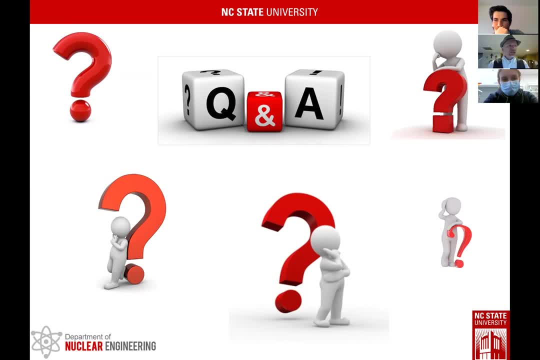 And so in a day and age when I mean think of this was over 100 years ago, Almost 120 years ago- The ability to what looked like and actually was curing cancer, We still do it today With radiotherapy, And so with that, people started verifying that you actually could do that. 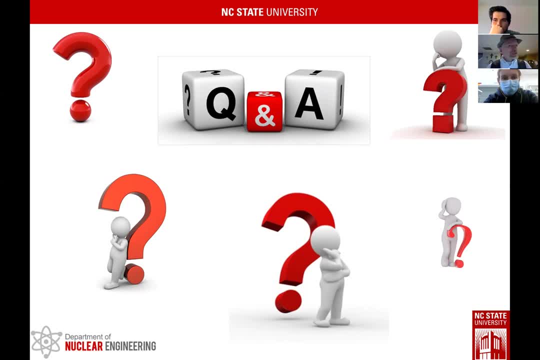 But what that led to remember the level of technology that they had back then. It was like a miracle drug So that people would be drinking radium salts. It wasn't until we had the radium dial painters that we realized that this stuff could kill. 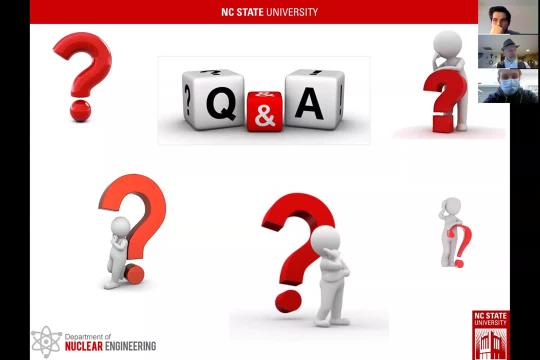 And that was that they would take radium and they would put it in paint, And they would paint the dials on watches, where the paint was glow-in-the-dark paint, but it had radium in it, And so the dial would always show. 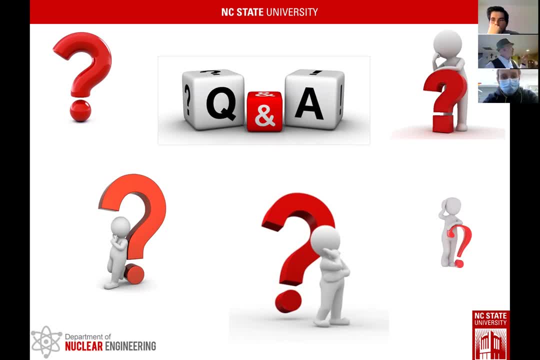 It would always light up like an exit sign. We used to use tritium in exit signs to keep it lit when you had no power, And so, because they kept doing that, they would wick the paintbrushes in their mouth And then that way they would have a very fine tip. 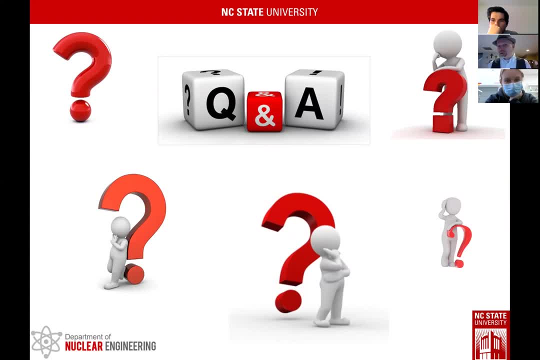 And that way they would paint the dials on there. Well, after about 20 years of doing that, they all got these horrific mouth cancers, And so it was like: well, how can this radium, which cures cancer, cause cancer? 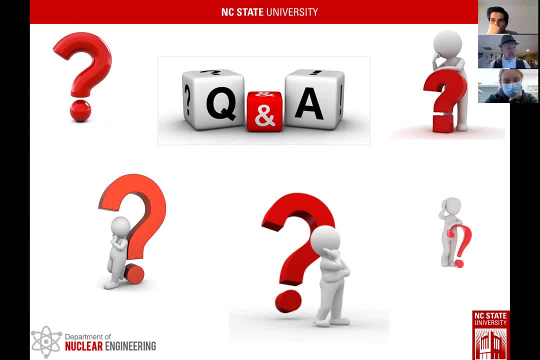 Well, that's because not only does it kill the cancer, but it can also cause damage to the tissue if it's in a very large dose. And so the applications before that were this idea that it was a miracle drug- right, It was this miracle of science that was very highly attenuated once they realized that at large doses this can kill. 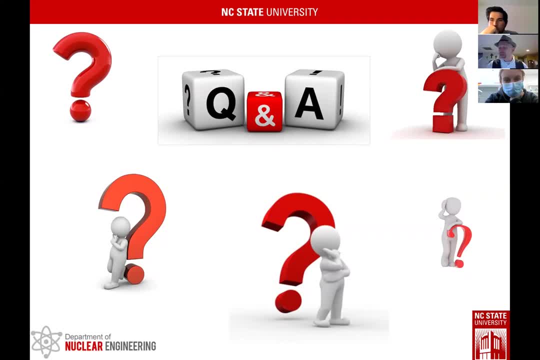 In fact, many think that that's how Marie Curie died was because of this lack of knowledge of the effects at high dose that they can accumulate if there are these acute doses. So there were a number of things that were like that before the Manhattan Project. 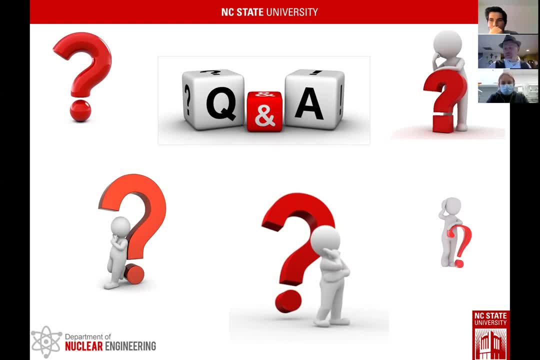 And for the most part, though, it was a research topic and people were still trying to figure it out, But that was probably the biggest one was- it was very early- recognized that this could be used for medicine. Well, Lord Rankin- what we actually named the Rankin for- recognized that you could see through a hand. 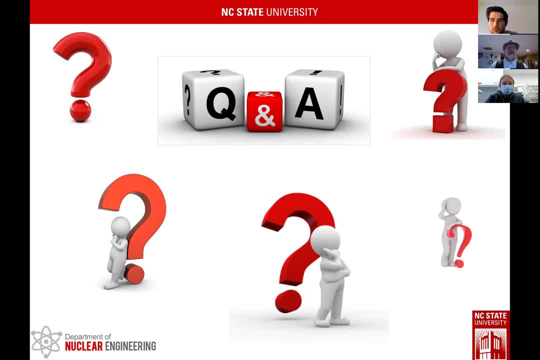 Right, If you see a broken bone, you know I can do a lot. I hope that answers the question. And they also make to used to make old glassware out of uranium. So they did for a long time And even after the Manhattan Project. 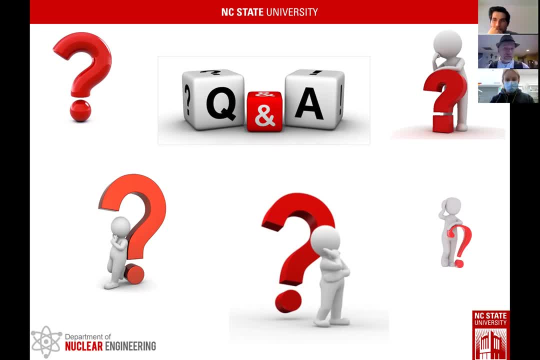 But that was with uranium compounds because it gave very fancy colors. But what ended up happening is that 20 or 30 years ago people just like lantern mantles, people would use those to do demonstrations for the public. Like put a Geiger counter up to it, make the thing scream. 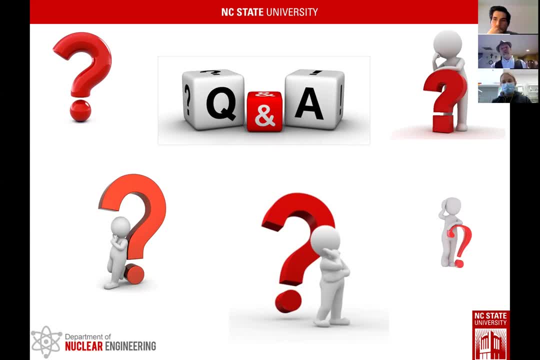 And that would terrify people, even though they were trying to say: look, it's harmless, This is not a big deal, This is natural stuff, And I just put some dirt and I put it in some and I and I centered it and I made it a glaze. 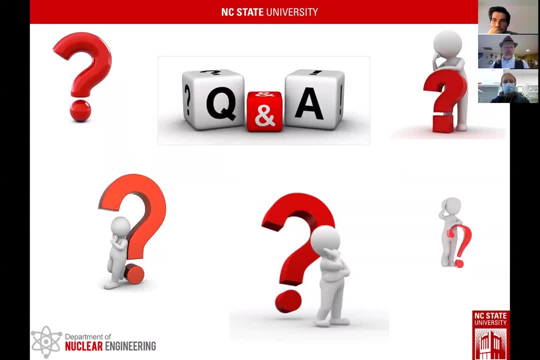 But now it makes the Geiger counter, you know, 10 times higher than it is when it's away from the plate. And yeah, it's 10 times higher back there, right there. But at background again, you can go over large variations without an order. 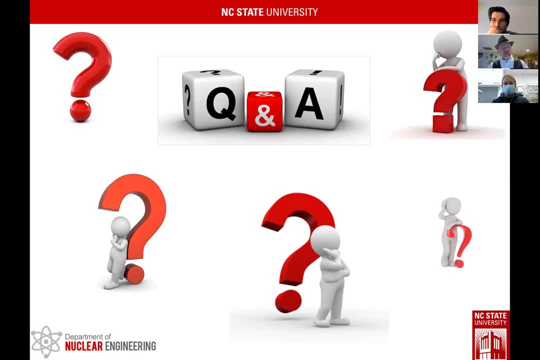 Magnitude of background with no measurable effect. actually a little bit more than that, But without communicating that. it just terrified people, So they actually banned the use of that. Oh, I don't know about 10 or 15 years ago, using uranium blazes to make Fiestaware. 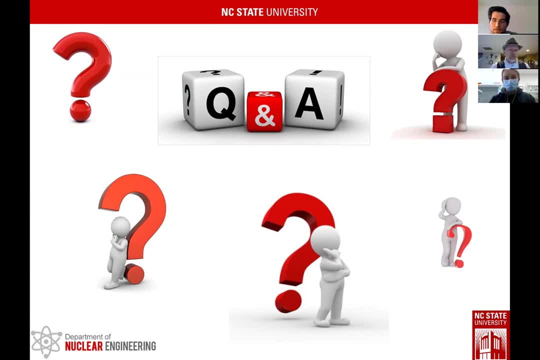 That's what it was called, And the same with lantern mantles. Those used to have thorium and thorium oxide to help it from not burning. So they found other compounds again, simply because of the fear of naturally occurring radioactive materials. We have another question from Mr Braden Goodwin. 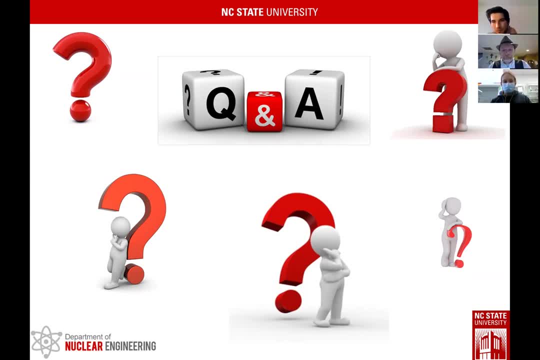 They want to know when were these workplace REM, millirem, regulations and limits put into place in the US, And were the specific values that we use today still derived from events such as the atomic bombings or any accidents? So we actually did have regulations all the way back till, even a few years before the Manhattan Project. 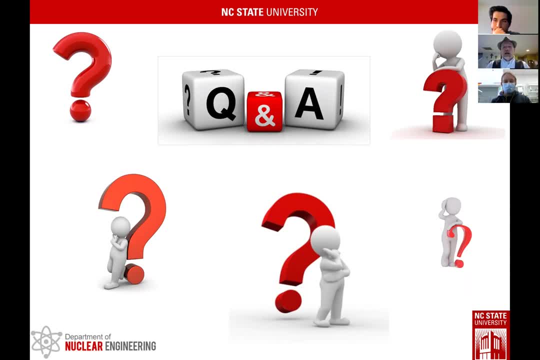 So that they actually had limits. But the limits back then were substantially higher. If you look, if you remember, back to that risk table, they actually reflected those risk tables so that they said, unless you get a measurable effect, we're not going to worry about it so much. And so it wasn't until substantially after that, right around in the 70s, where the limits we have, where we're saying we're not going to let people even be exposed anywhere near a measurable effect, We're going to cut it by at least an order of magnitude, and sometimes even more, a few orders of magnitude. 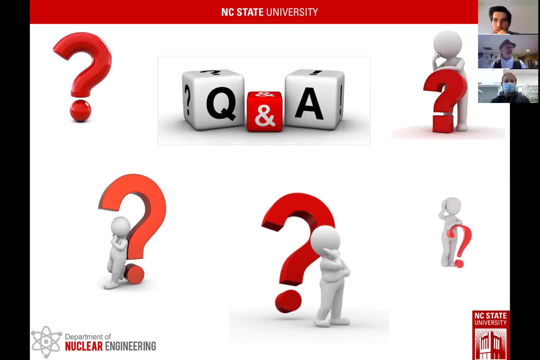 It's got to be even less than backwards, And so that started around in the 70s, where that level of conservativism was built into our radiation protection regulations, which, even though it's ultra conservative, people tend to interpret: if it's a regulation, then that's the only thing that's safe. 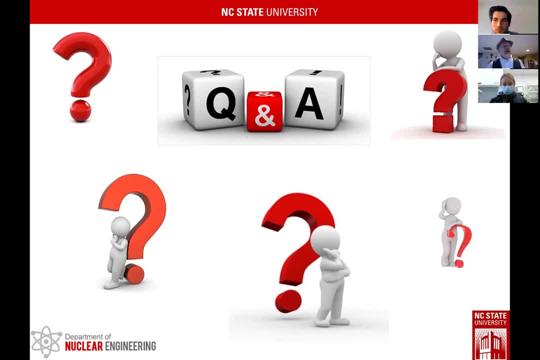 And if that's safe, I want to be even safer than that, Even though that's already built into the regulation- that you're substantially below a measurable effect, Which, In the case, for example, even with through Fukushima, like it was with Chernobyl, the psychosomatic effects turned out to be the deadliest, and so I had it in the slide. I didn't point it out. 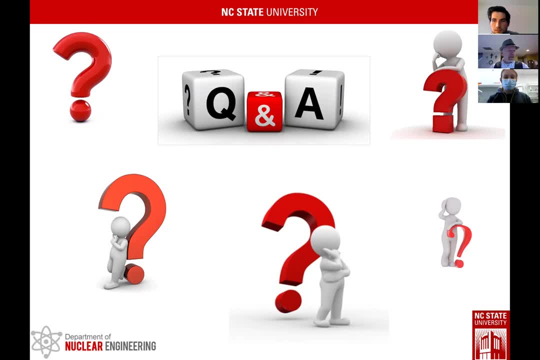 The only deaths from Fukushima were from the panic evacuation. It was in the slide that I had. there was a reference there- But the point is is that people literally risk their lives and lost them to avoid something that wasn't even measurable, And that's kind of that. That's why there's this emphasis on recognizing the effect of radio phobia like a curse. right, if you believe it, it can become, it can affect you. 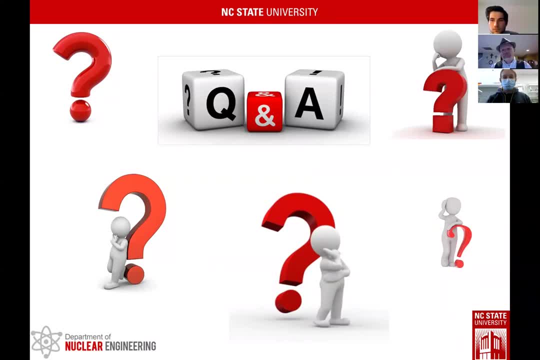 If you believe it, even if it's just words. Um, AJ Benny wants to know: how is the Q value determined in that dose equivalent formula? So so that comes from historical studies on things like radiation, Historical studies on things like animals, so that you recognize that if cells are replicating, if you have stem cells and you're radiating them, then they're more likely to have a measurable effect. 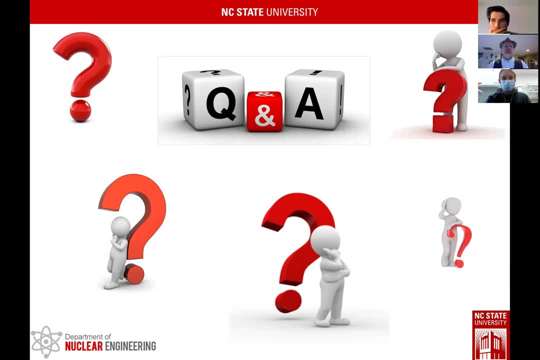 So when they're, when the cells are proliferating, for example in the first trimester, If you have a fetus, that will get a dose, say around 100 rim. it's a huge dose. It is likely going to cause a defamation abnormalities. there's a it's kind of like fetal alcohol syndrome. 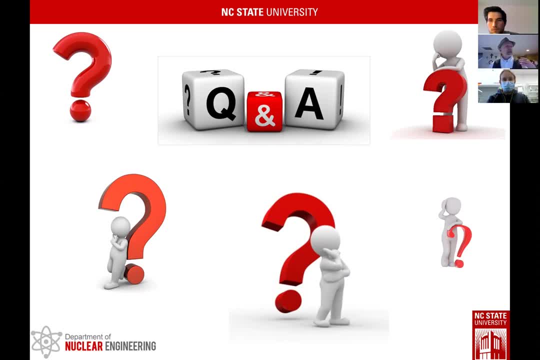 Right. if the female is an alcoholic in the first trimester it can cause birth defects. And those large doses will also cause birth defects. they're not genetic, So the gene isn't changed, but the development of the fetus is stumped because the cells are proliferating. And so you know, if you have a fetus that will get a dose, say around 100 rim, it's a huge dose. If you have a fetus that will get a dose, say around 100 rim, it's a huge dose. 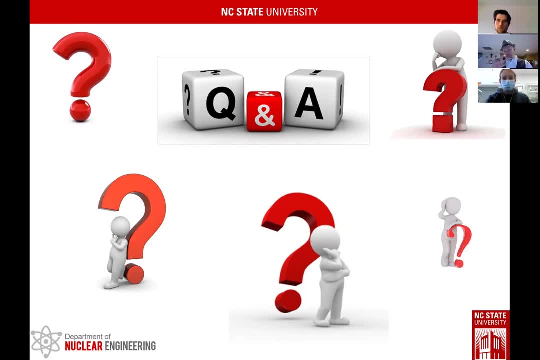 And so, in order again to mitigate that, there were, when I looked at, when I had that, the regulations table, that actually had a lay, an entry there for a pregnant radiation worker And that's even lower than a regular radiation worker And that's many orders of magnitude below what would actually cause a measurable effect. 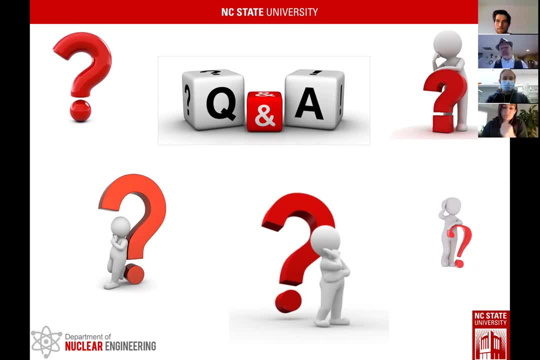 And again, let's just put this level of conservatives- conservatism that's built into the regulations. Hope that answered it. two questions from Zachary Miller. The first: do you think fusion, if possible, would be safer from a health physics perspective than fission? No, So fusion actually also causes radioactivity. 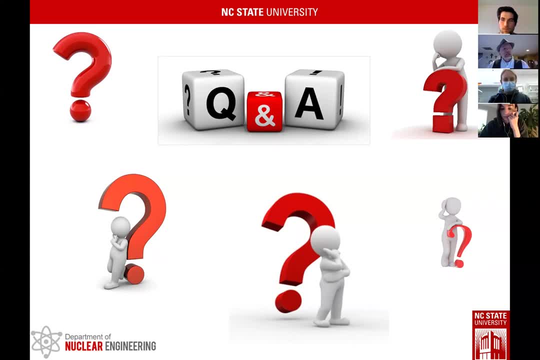 It would be like. I mean, the analogy is like: is making aluminum safer than making nickel? If you make it safer, then it's safer. If you don't make it safer, then it's not safer. So it just comes down to how you do the design. So I like to quote Forrest Gump: safety is as safety. 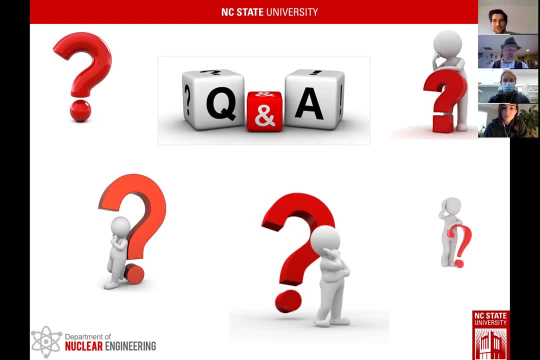 does. It's up to you to implement a level of safety that you think it warrants. That would be my opinion. And the second question is: could you explain the salty disk joke before the presentation for a non-nuke major? Oh, yes, So the point is: is that they're not going to know if 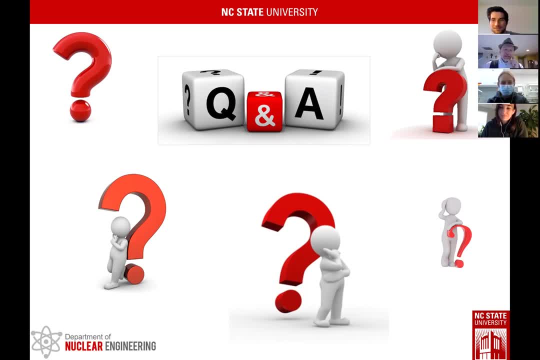 it's salty unless they touch their tongue to it, And if you're tasting it, that means that you're ingesting some of it, And if you're ingesting some of it, that means you're knowingly eating anthropogenic radioactive material. It's like 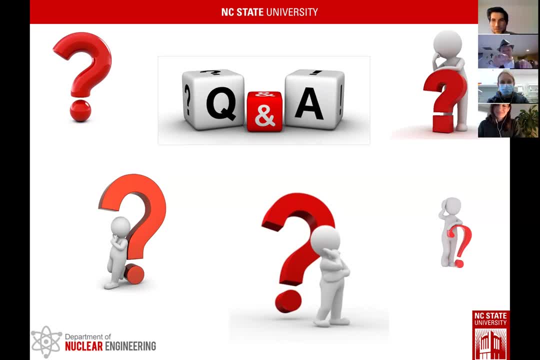 why would you do that? You're ruining the source on top of it, right? You're not putting thumb prints on it. You're putting tongue prints on it, And it's just a bad practice to think you can go around doing that, because you don't even know how much radioactivity you're taking in, right It's. 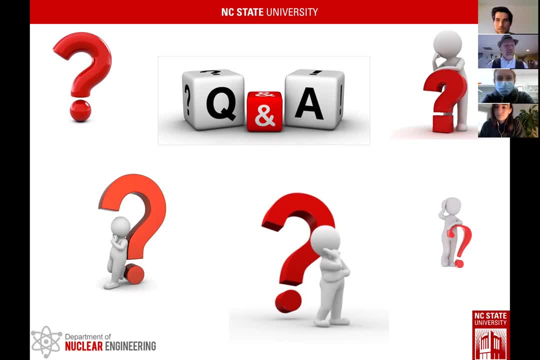 kind of like the radium dial painters. We know if you get a lot of it it's going to cause a problem. How do you know you didn't get a lot of it? Did you even take a measurement? Did you measure before and after? Do you know what went into it? Apparently you didn't even care or you wouldn't. 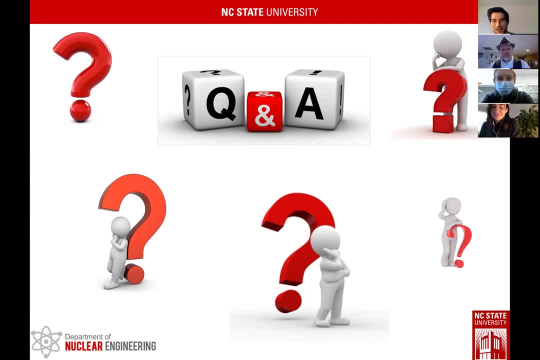 be tasting it in the first place. And then I think we have time for one last question. An anonymous attendee wants to know what is the best valid argument against nuclear energy from a health perspective. It's the radiophobia. So it comes down to. 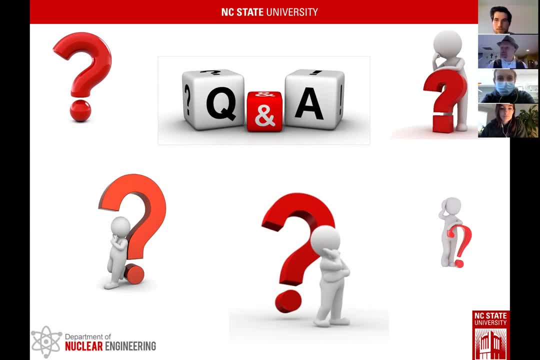 if I told you that you're cursed and you believed it, then you're going to stress and you're going to reduce your immune system, and your reduced immune system is going to make you more likely to have a health effect. If you have a health effect, you're going to attribute it to 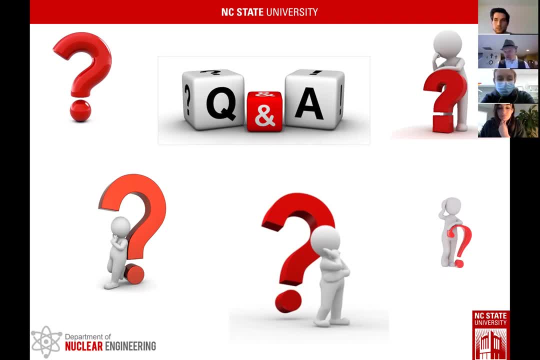 the curse. And so you're going to think, oh, I'm cursed, right. So that's why the number of deaths from Chernobyl have been the dominant number of deaths are from suicide, from people that feel they're cursed. Everything is just going wrong, And so the same has actually occurred with Fukushima. It wasn't so. the health effects: the main health effects are the deaths from the evacuation, But the follow-on health effects are the deaths from the evacuation, And so the health effects are the deaths from the evacuation, are again from radiophobia, It's hypertension, it's stress-related heart disease and 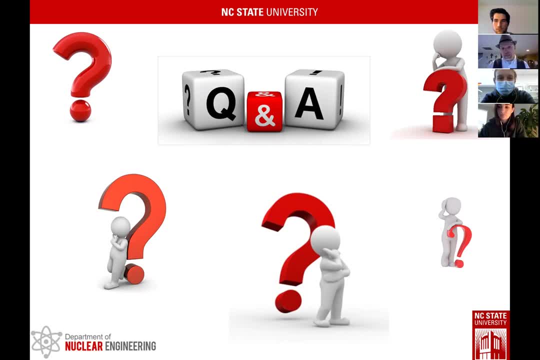 diabetes from overeating. So what they found is that- I mean, unless you're going to say, well, even if you're afraid radiation is going to cause you to overeat because you're stressed, that's really not what the professionals say. That doesn't make sense. What does make sense? is that you think you're cursed. If you think you're cursed, then that causes you to stress And that stress is a measurable does give a measurable health effect. It reduces your immune system, So opportunistic diseases are easier to get a foothold and take you down.